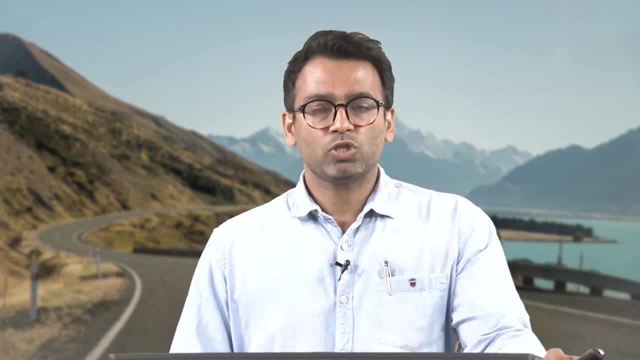 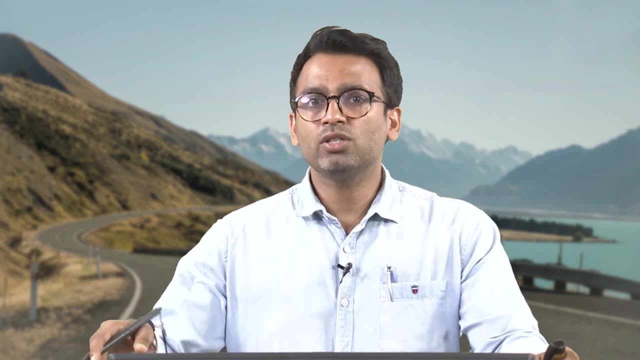 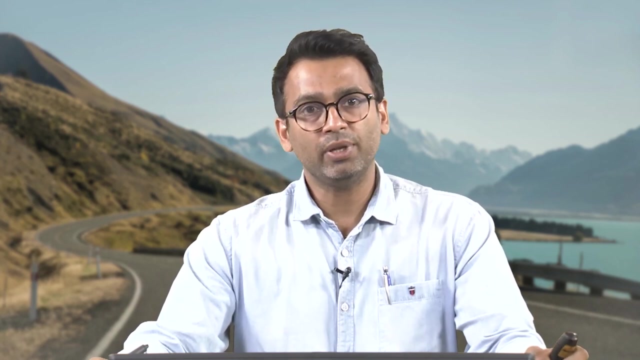 Today we will also touch upon the topic of soil, which is the first pavement material we are going to learn in this particular lecture module. This course in general is meant to expose you to various fundamental concepts related to the use and application of different pavement materials that we use in pavement construction. 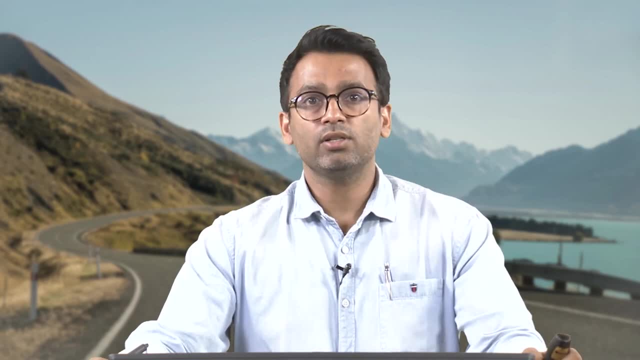 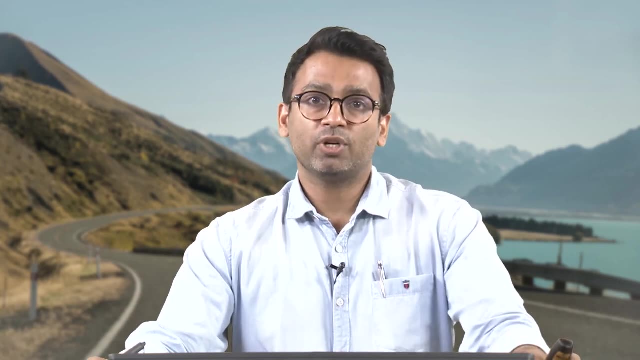 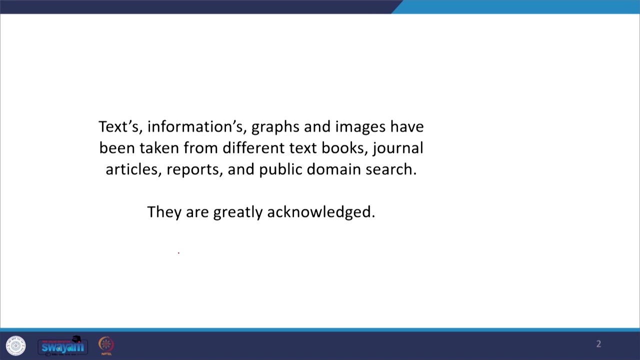 I hope that this course on pavement materials will be useful to all of you, specially those who are learning this particular subject from the perspective of their course curriculum. Before I begin, I would like to inform that this text, information, graphs and images that have been used to make this lecture and. 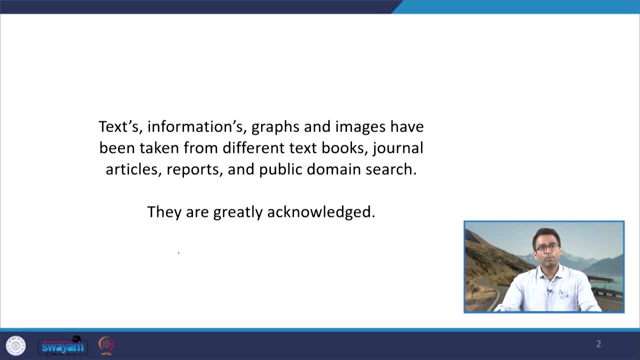 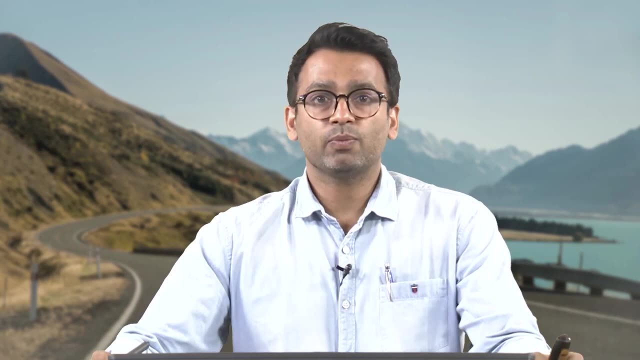 other lectures as well in this particular course have been taken from different text books, journal articles, reports and general public domain search, and I greatly acknowledge them. Now, since this is the first lecture and we are just going to start talking about various aspects of pavement materials, I would like to take this opportunity also to thank my 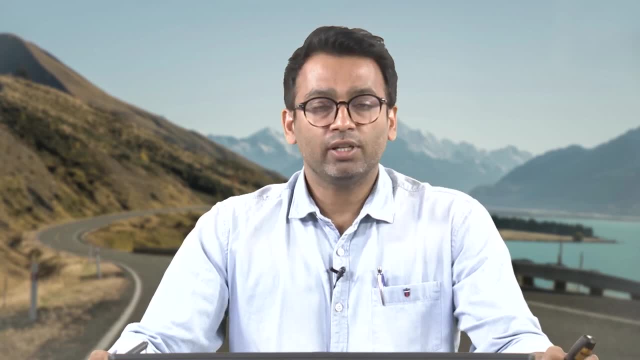 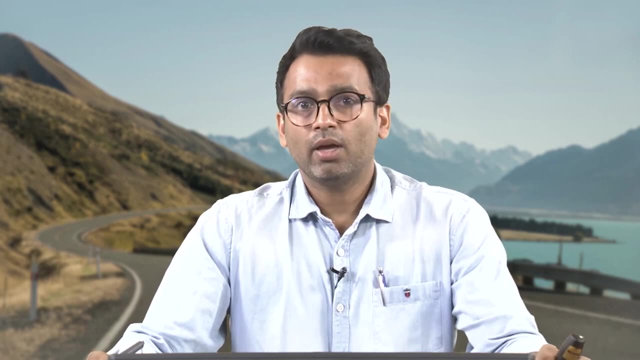 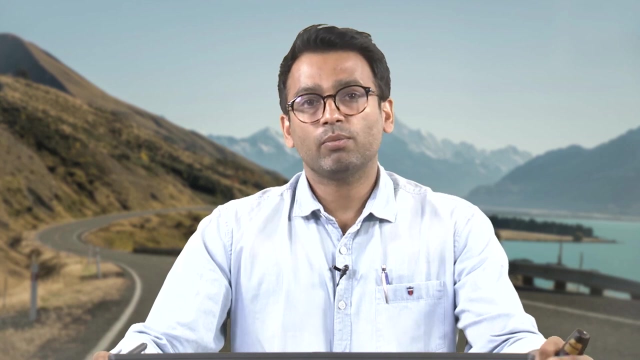 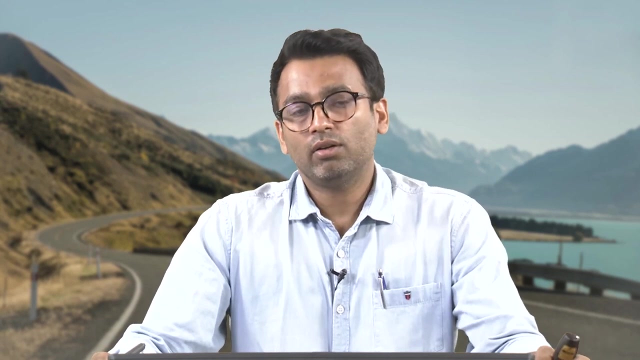 teachers. My teachers were my colleagues from different institutes and also my students In general. various discussions with them have greatly enriched my knowledge, ah in the area of pavement ah materials, and also this process is continuing with time. I also would like to thank various other lectures on pavement materials that are available in 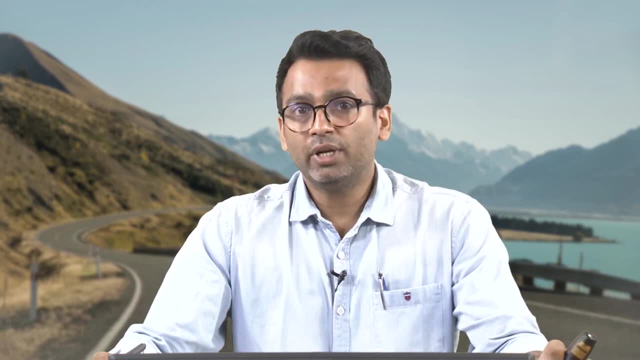 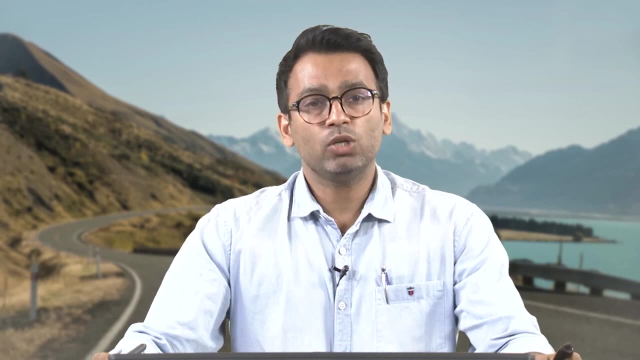 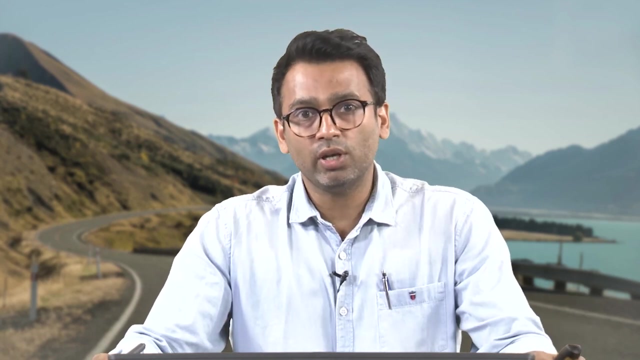 public domain. there is an NPTEL ah lecture by Professor K S Reddy from IIT Kharagpur and I feel that you know these lectures are very useful and my lecture, or this particular subject which we are going to learn, is just an addition to the existing knowledge in the area of pavement. 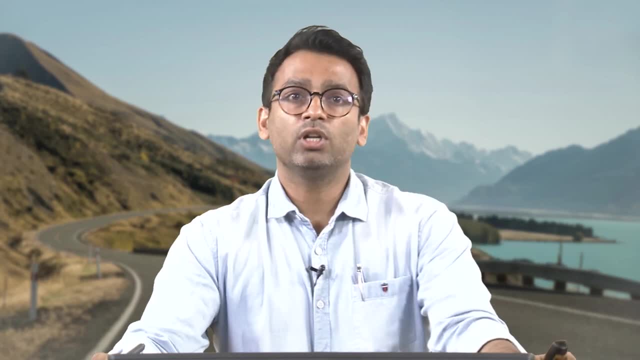 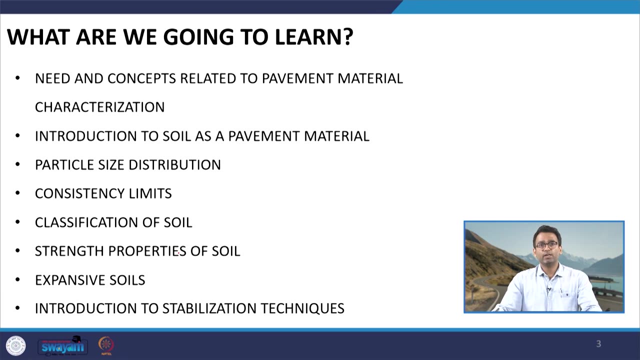 materials. So what are we going to learn in this particular module? We will talk about the need and concepts related to pavement material characterization. So this is just an introduction to the subject. We will also talk about the introduction to soil as a pavement material, As I mentioned. 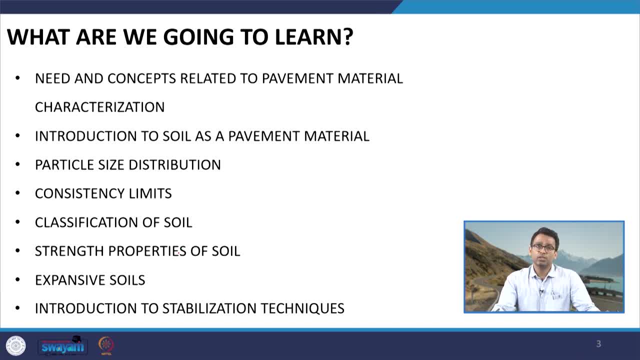 soil is the first pavement material we are going to learn about in this lecture. We will also further talk about the importance of particle size distribution for soils. We will learn about various consistency limits, for example liquid limit, plastic limit and the use of plasticity index. 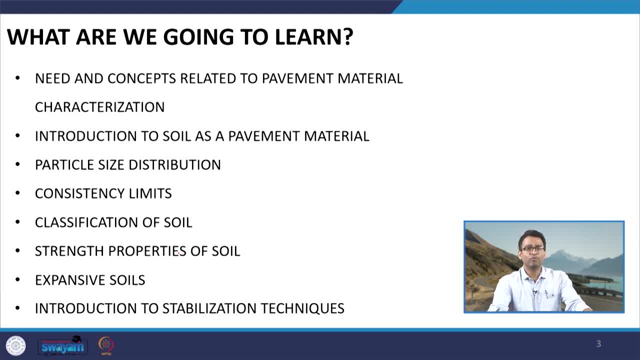 We will also talk about briefly about the use of plasticity index. We will also talk about the different classification systems for soil and we will ah spend some time to discuss about the classification system we use in India. We will further explore the various strength properties of soil that are required to study pavement as a system. We 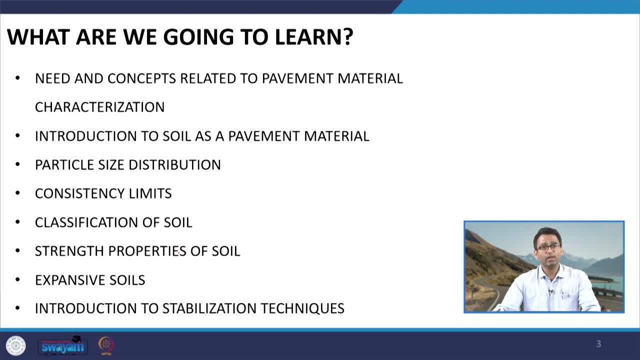 will talk about the expansive soils, which are very critical soils, and we will further talk about the various ways to stabilize some of the soils which, in general, we are going to discuss in this lecture. So let us begin with the introduction to soil as a pavement material. So let us begin. 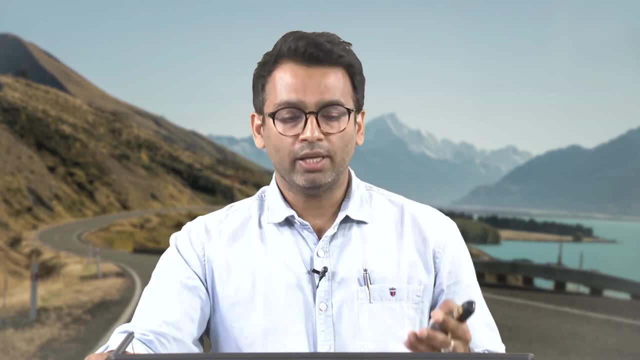 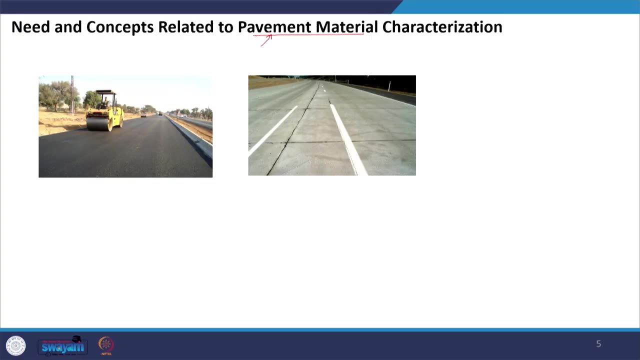 by understanding the term pavement material. So when you see the term pavement material, we have a predominant term here is pavement, So we are learning about materials that are used in pavement. So just to begin, just to- ah, you know, have a feel about this subject. 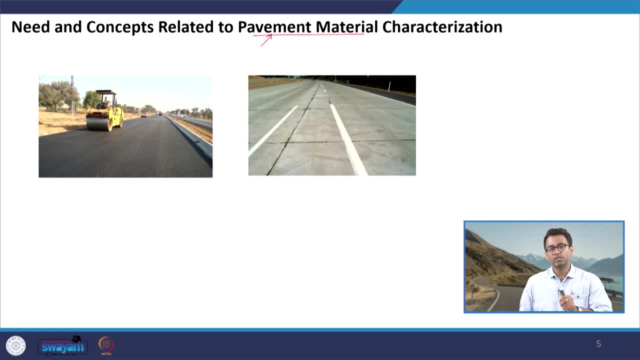 let us try to see the two basic pavements that are, you know, typically used in construction. So we have a flexible pavement here and we have a rigid pavement here. So these are the general terminologies. So, as you can see, some of the differences you can make out. 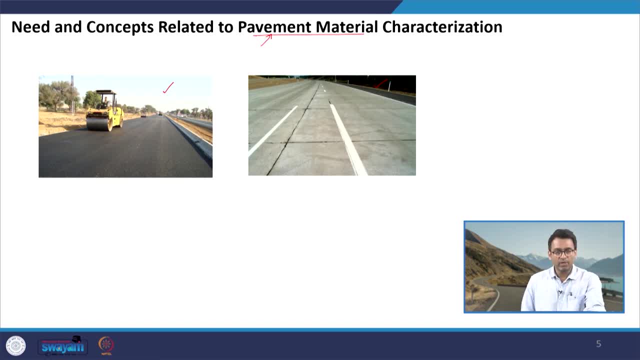 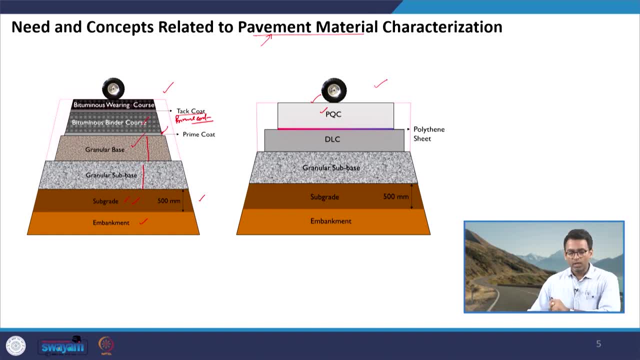 application tack coat. So we put a tack coat and then we put a bituminous wearing course. On the other hand, if you see the cross sectional element of a concrete pavement again, the lower part remains the same. that is, we have embankment and we have subgrade, above which we are going. 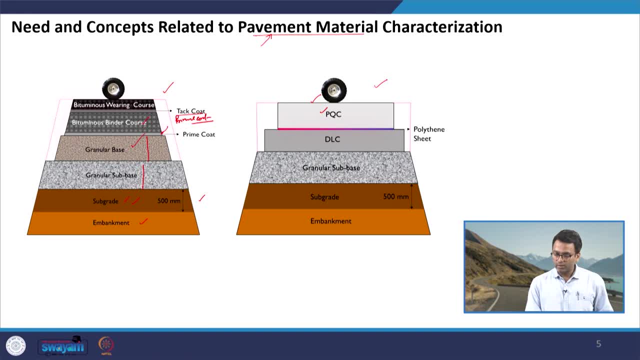 to construct other layers, Typically in concrete pavement. the need of other layers are not specifically so important because the concrete slab itself has the ability to take off most of the load that is going to come on the surface. However, because of other criteria's for 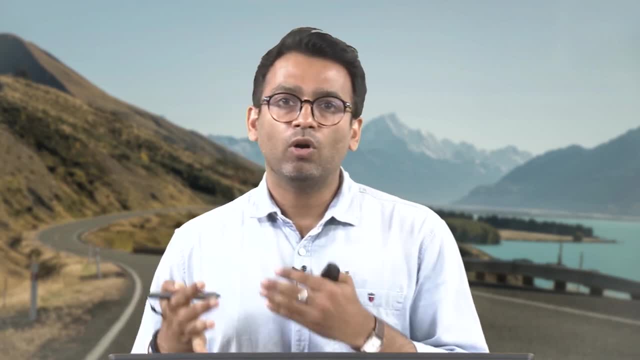 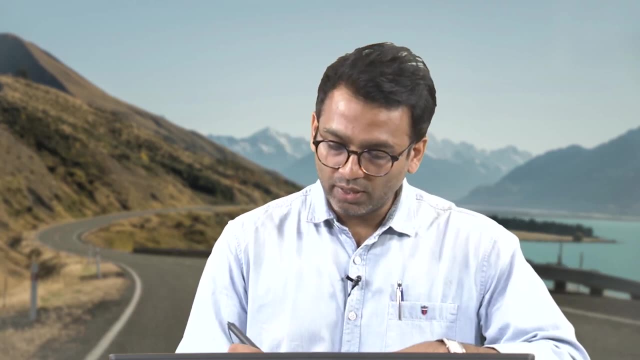 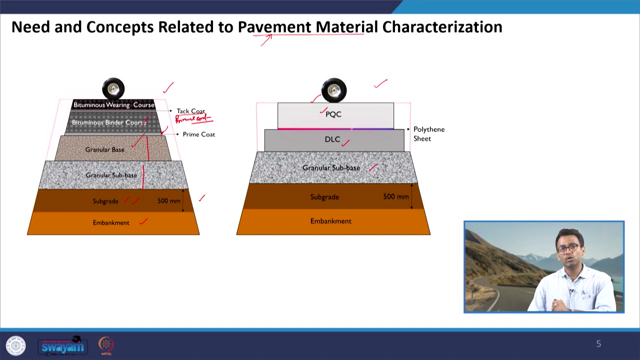 example erosion of ah layer below or permeability requirement. other layers are also used in the construction of concrete pavement. For example, we have a granular sub base here, above which we put a stabilized layer, typically which is DLC or dry lean concrete. then we put a polythene sheet to eliminate the friction between the. 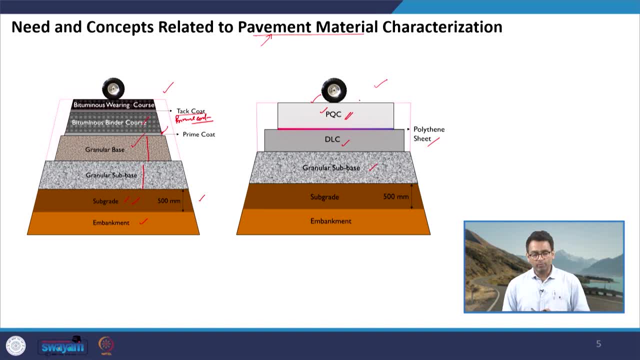 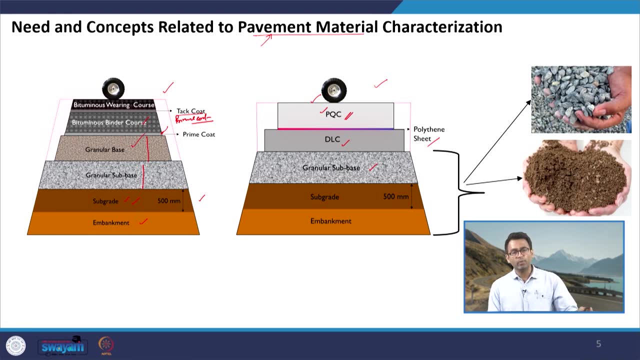 two layers and then we have the PQC, or the pavement quality concrete placed at the top. Now, if you see the materials that are used, you know, to make up all these layers. So let us see, ah, the materials that are typically used in the common part in both the pavement. 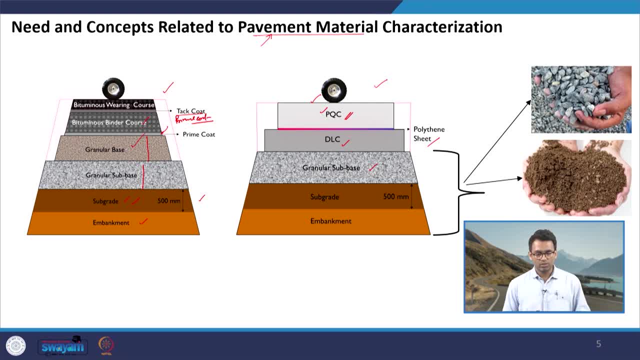 that we have embankment subgrade and then we have granular layers, So up to the granular layers. So we have either the natural soil that are typically used in embankment and subgrade and then we have granular materials that are used for construction of granular sub base. 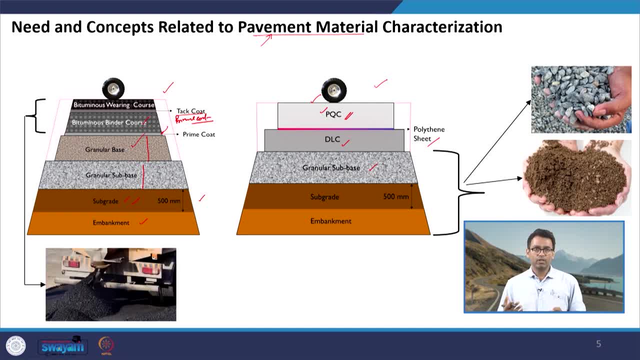 and as well as granular base, The bituminous layers, on the other hand, is basically a mixture. So this is a mixture of aggregates and bitumen, all right. and then, ah we, we heat the aggregates and bitumen together, we prepare the mix, and this mix is further laid for the construction. 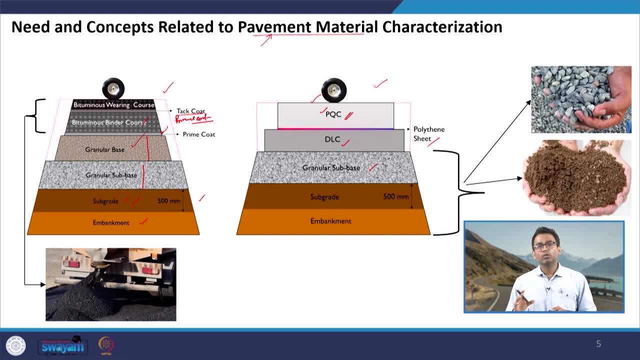 of the surface layer In a flexible pavement system. Then we have on in the concrete pavement. we have dlc and pqc. both are made up of cementitious material. In dlc the amount of cement is considerably less in comparison to PQC, but we can try to imagine both this material as a concrete 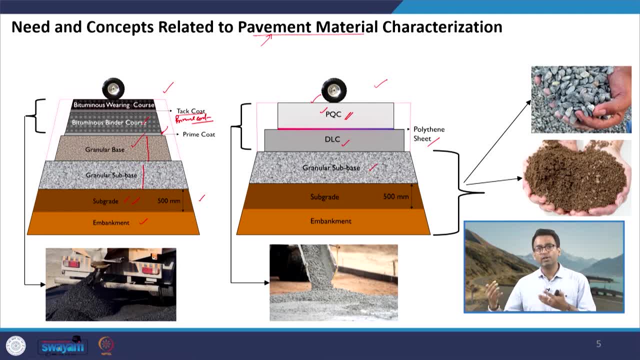 mixture. So we have cement, water, aggregate, sand and other ingredients that are mixed together and then that are laid and then these layers are compacted. So you know, before I begin to you know, further slides and because we are able to see most of the materials here. 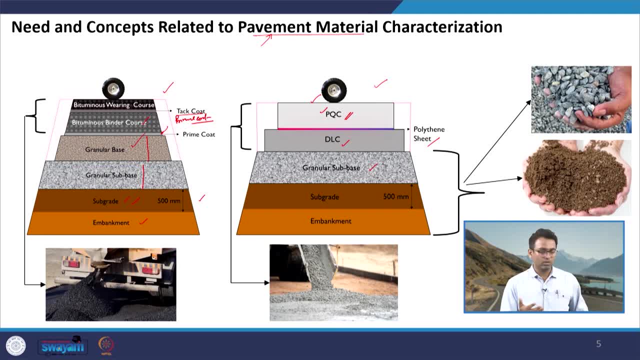 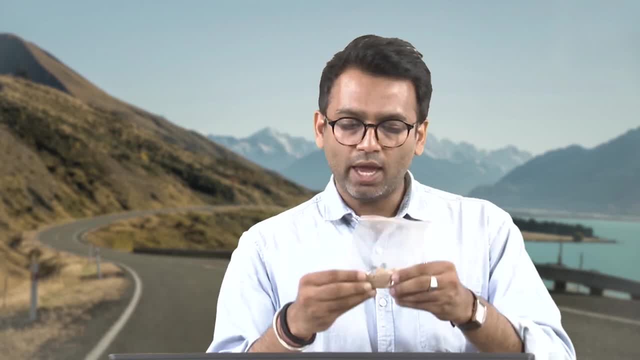 and we have talked about it. let us try to see these materials with our eyes. So here I have today with me, because we are also going to talk about soil, So I have, you know, different types of soil. you can see that I have. this packet is a type of soil. 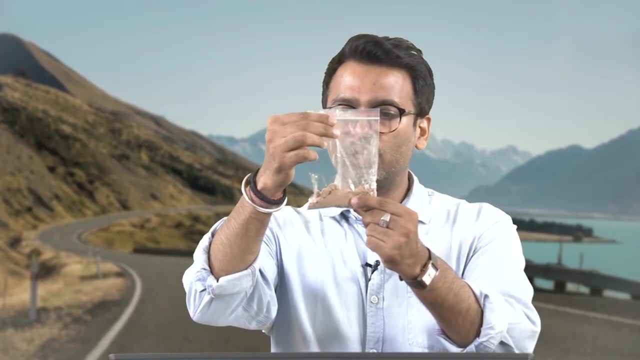 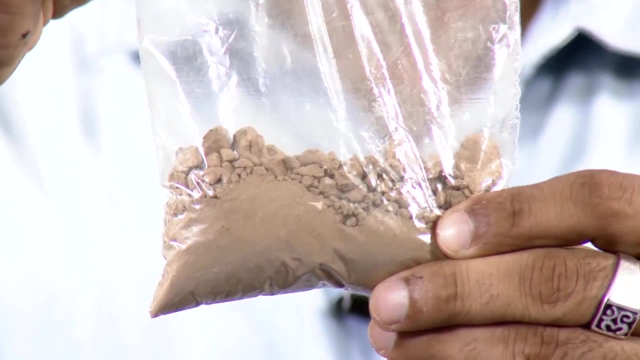 it is more of clay in nature, not very much recommended for the construction of foundation and pavements, but this is a type of soil. This is again another type of soil, a little darker in color in comparison to the previous packet which I just showed you. 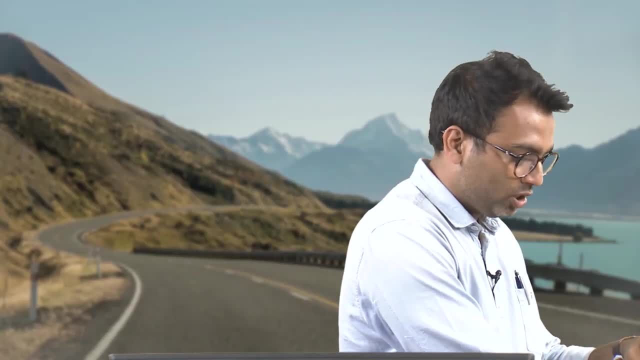 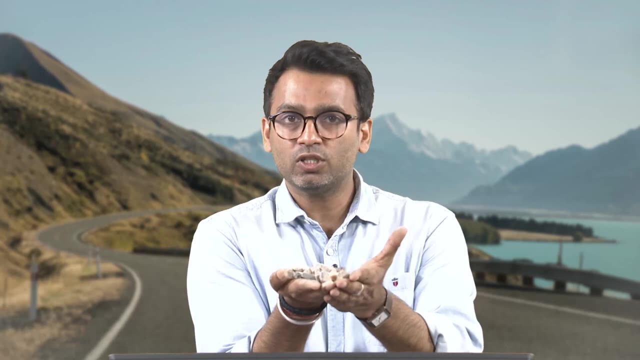 We also have aggregates here, as I mentioned that. this is used for the construction of granular layer. this is used, you know, for the production of bituminous mixtures, concrete mixtures and so on. So these are some aggregates in my hand, though these are single sized aggregates. 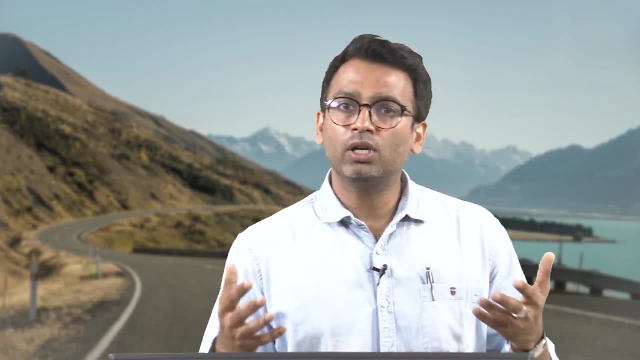 which I am showing you presently. But in practice, in a particular layer, the aggregate is there. So if I have this layer and I press it and then I move it, that this brigades can be present in various different sizes depending on the target gradation. We 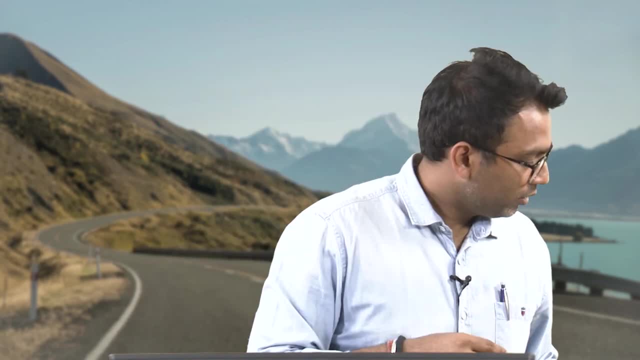 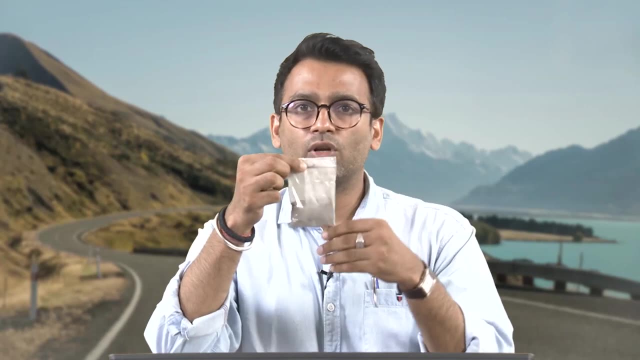 are going to talk about these aspects as we move forward. Then we have a packet of cement, So you can see that this is cement that is used for the production of a concrete mixture or a dry lean concrete mixture. We also have bitumen. 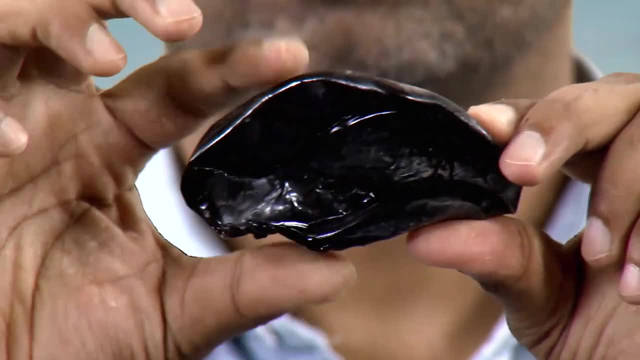 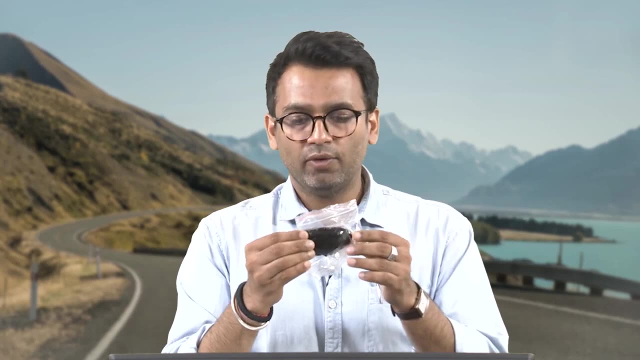 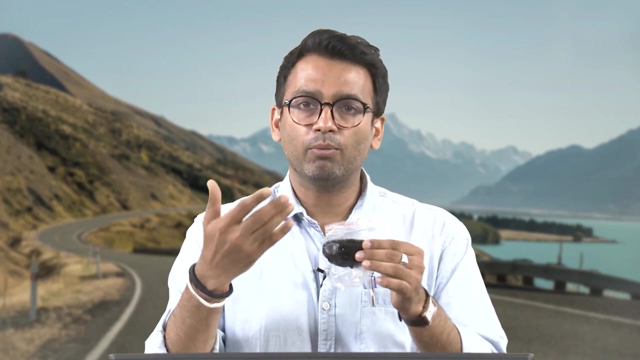 So this is mostly I mean now. it is more of semi solid in nature because the temperature of the room is around 25 to 26 degree Celsius. but if you heat it, this will become fluid, and if you cool it down it will, you know, become solid in nature. So this is more of a viscoelastic. 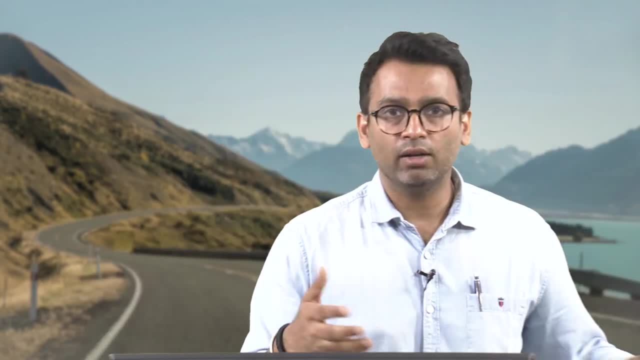 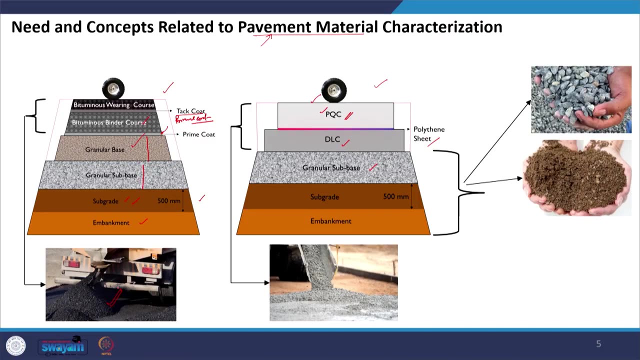 material, and we will be discussing about this material in detail in our lecture series. Then we have a bituminous mixture here, So this mixture is something which you can see in the picture here. So this is the bituminous mixture, composed of aggregates of different 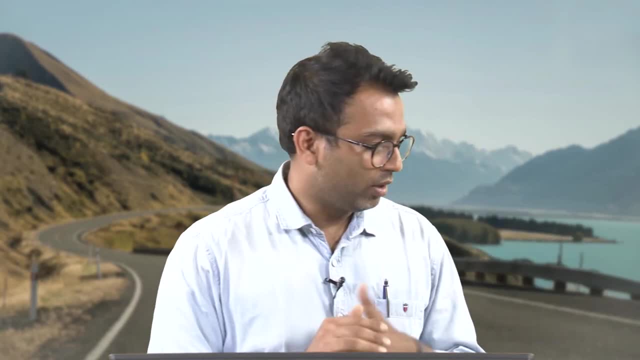 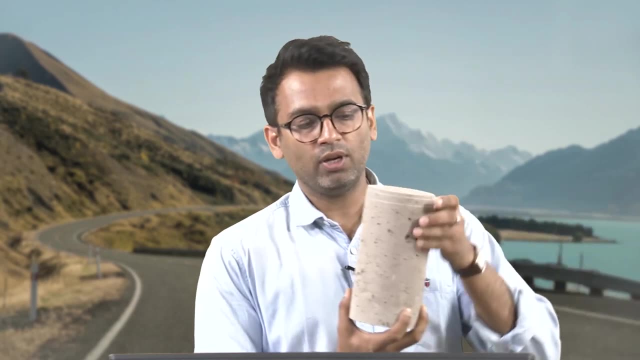 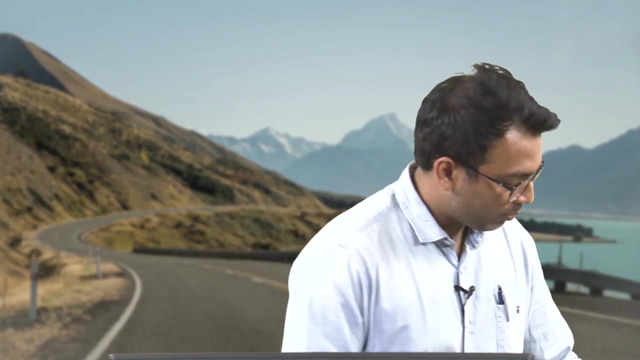 sizes And bitumen mixed together and we also have some quantity of air voids within the volume. This is a cylindrical sample of a concrete mix. We also prepare cubical samples So I have one cubical sample with me. So this is a cubical sample you can see for a concrete 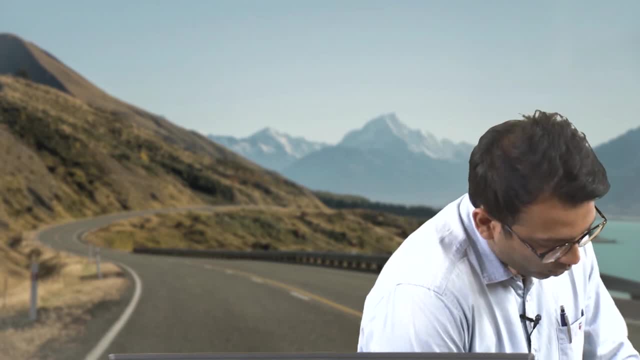 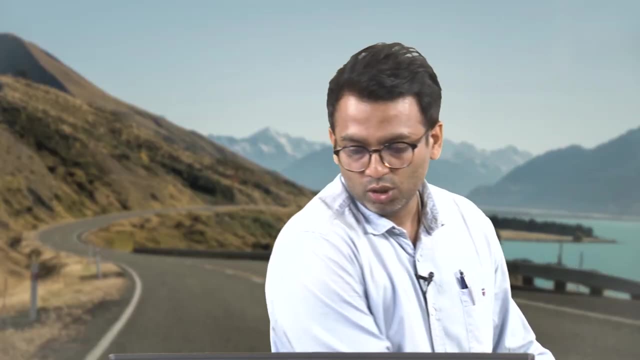 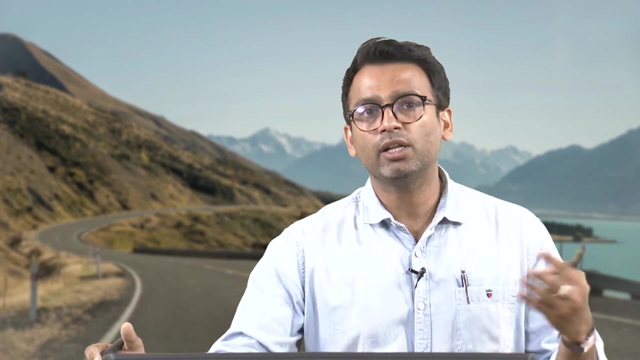 mix. The DLC is made also made up of concrete. you know cement based materials, but the quantity of cement is less. This was a DLC which I just showed you. So you know these are some of the materials. However, there are various other materials and my intention was to just to familiarize. 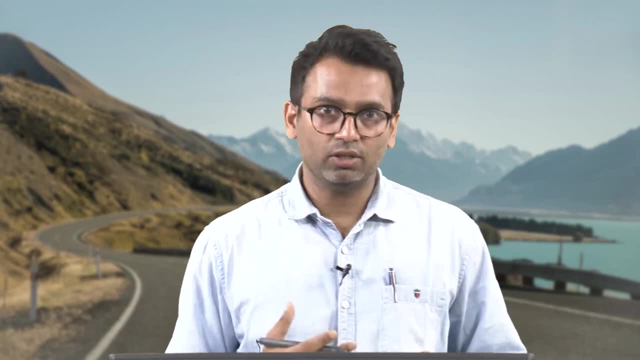 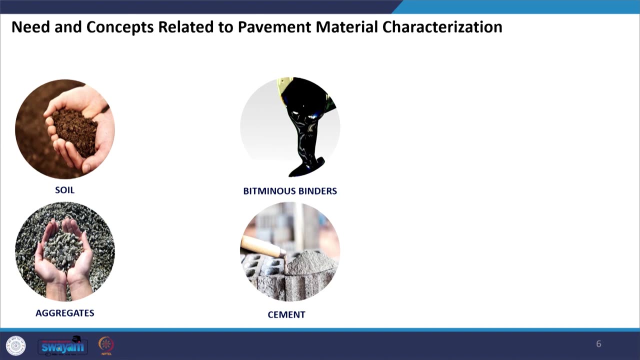 you with a visual idea of these materials. So some of the basic materials that are used in construction. it includes soil, it includes bituminous binders, aggregates, cement and there are various other materials, but these are some of the very 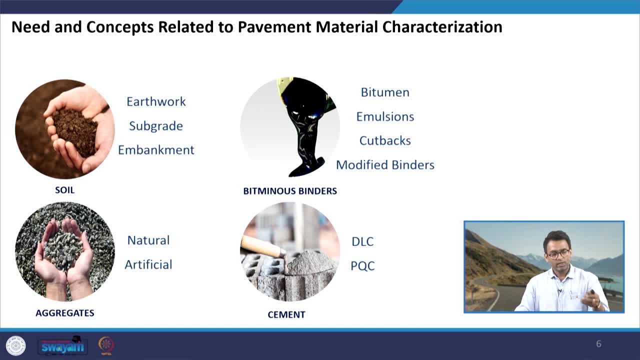 �� primary materials that are used.A would beisoil país. liketanoidMatster ontariéámatas arriéâmatas alive and clothingİち are used in construction for example soil is used in the construction or in earthwork 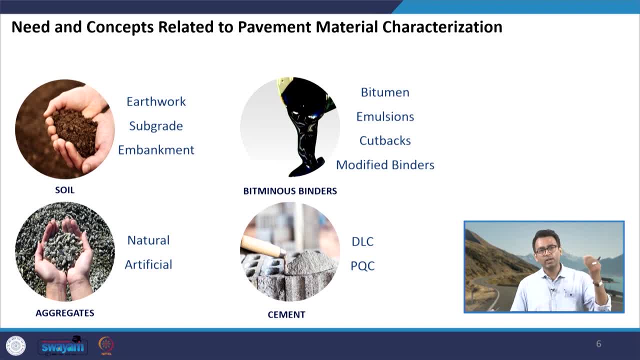 in subgrade, in embankment. aggregates are used in different layers of the pavement in different form. they can be from natural sources, they can be from artificial sources. for example, we can have industrial slag that can be used as a replacement of the conventional aggregates we have under the bituminous binders. also, we have certain categories, such as we have: 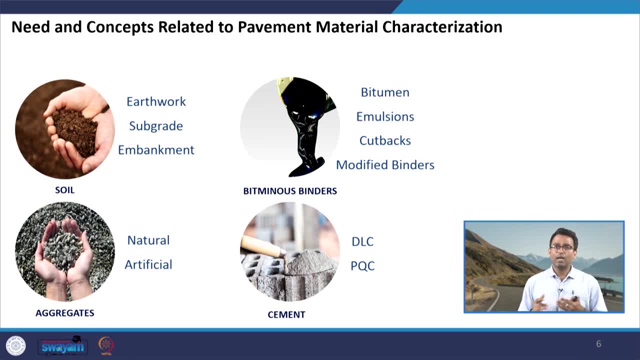 normal bitumen or viscosity graded ah bitumen. we have emulsions, we have cutbacks, we have modified binders. when you talk about cement, we have just discussed that this can be used for the production of dry lean concrete, for the production of pavement quality concrete. 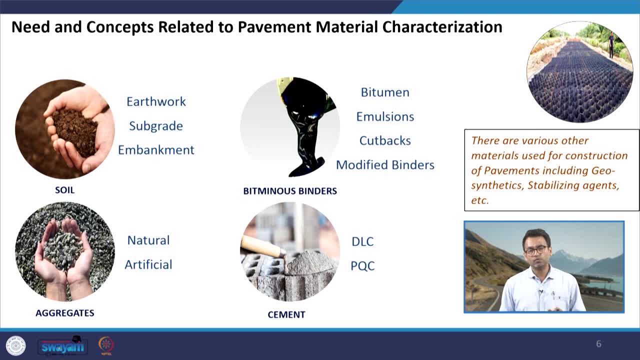 and so on. we also have other materials, for example geosynthetics, under which we have several products like geo cells, geo membranes that have been, you know, used in various pavement constructions we have. we have other stabilizing agents that can be used for stabilization of soil. we have. 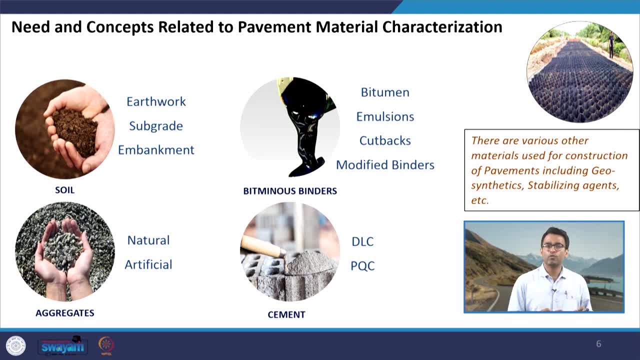 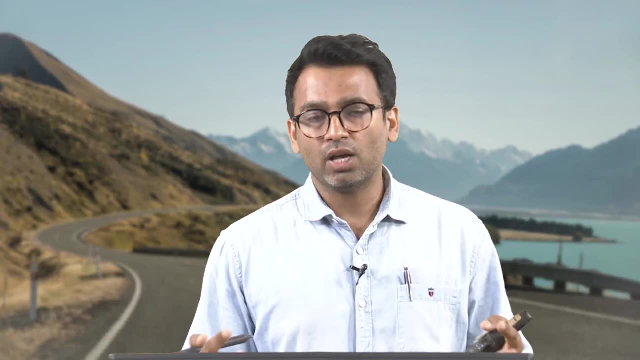 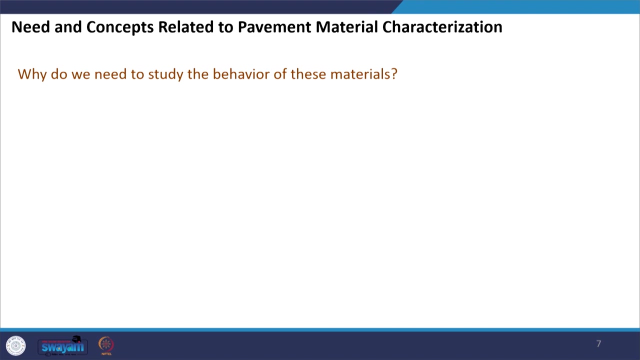 various chemical agents that can be used for modification of ah. you know primary materials. so you know, in pavements, presently the state of the art is that various different materials are being used, are being developed and in the future- you know this- numbers are going to ah, increase, ah in a huge ah range. now coming to the need of studying ah pavement. 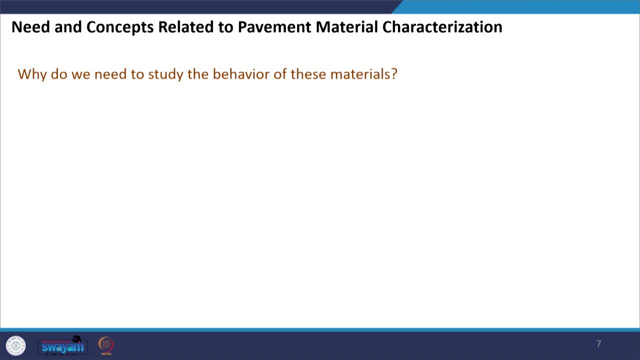 materials. so the question is: why are we ah interested to know about the properties of various pavement materials and why there is a need to characterize this materials before we can use it in the pavement construction? so there are various reasons which can be ah identified. ah that you know, that ah indicates about the need of ah studying pavement materials. one is to 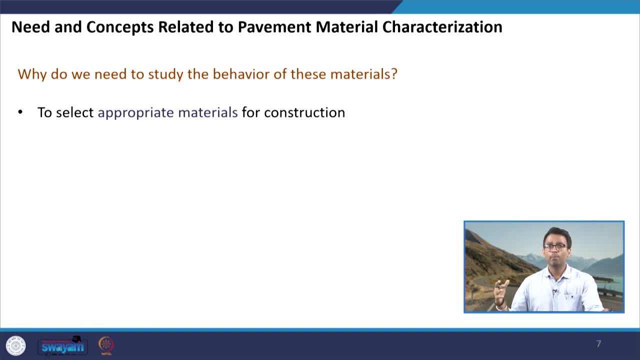 select appropriate material for construction. so this is like a pass fail criteria. so since, for example, we can have aggregates from different sources, these aggregates from different sources, different types, can have various mechanical strength, various different properties. now for a specific construction. i want that my pavement should be able to resist the load. 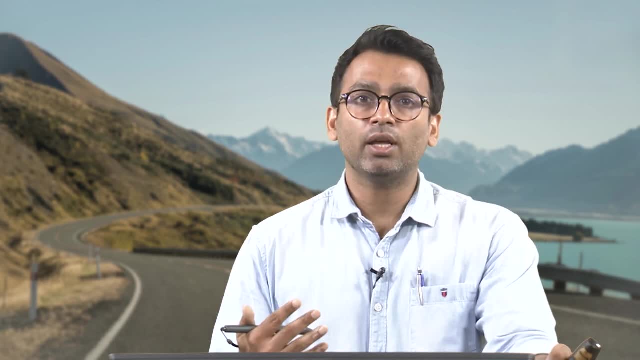 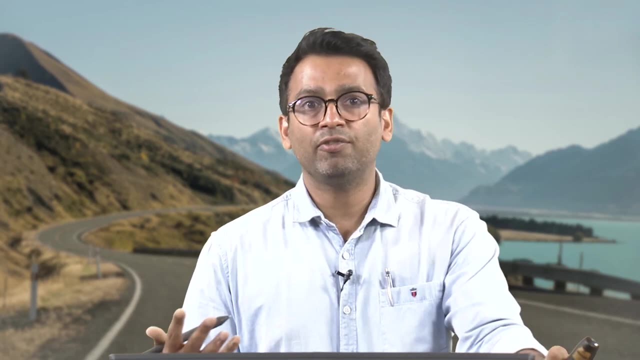 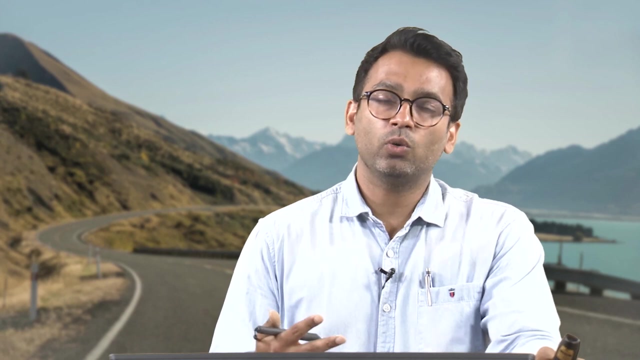 which is going to come. but if the strength of the material is very low such that it is going to take up the desired load, my purpose of constructing a pavement fails. therefore, it is important to me as an engineer that when i am, before doing going for the construction, 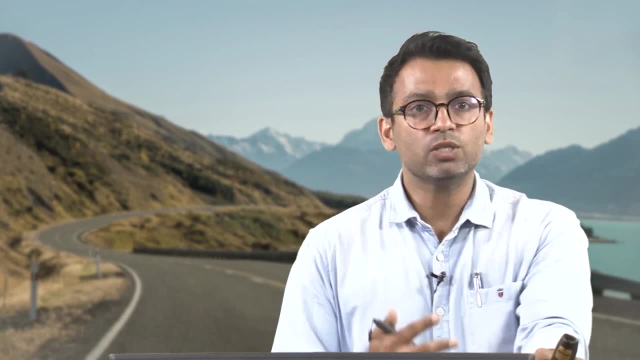 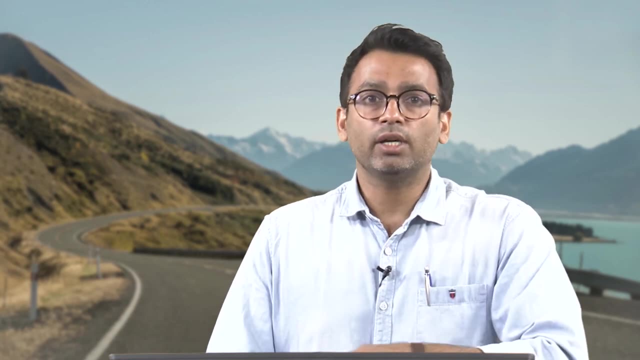 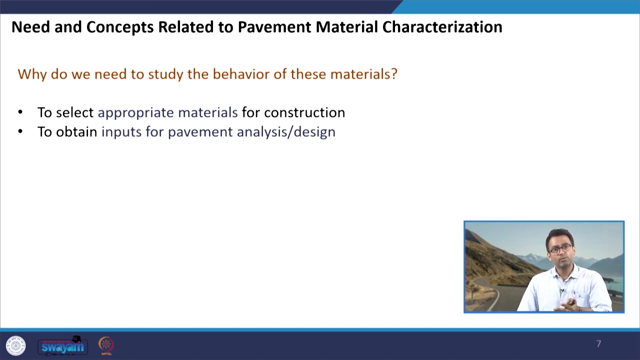 i have to test the appropriateness of these materials for the desired purpose for which the construction is being done. we also need to study the material to obtain inputs for pavement analysis and design, for example. let us say ah, for example, the material is going. if we are talking about flexible pavement design, in the flexible pavement design we use resilient. 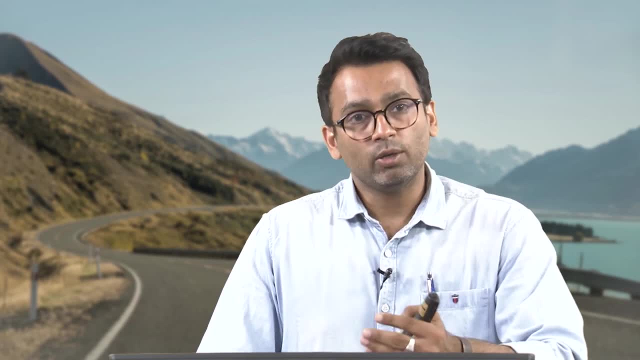 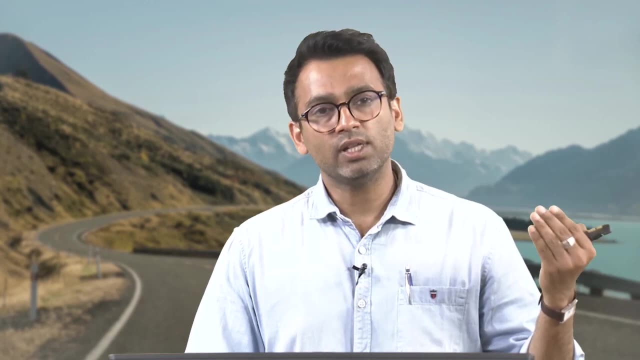 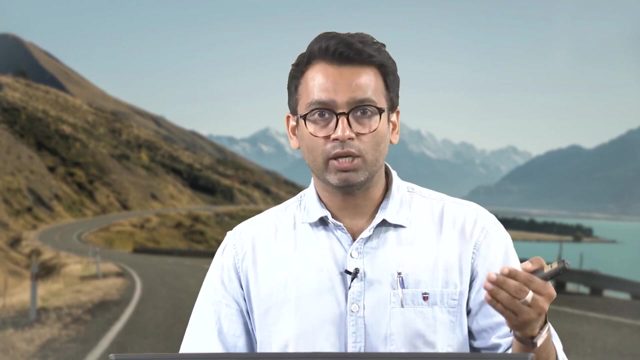 modulus as one of the properties for different layers. so that means that i have to have the value of resilient modulus of these layers in order to design the pavement, in order to analyze the pavement, in order to find the thicknesses of different layers for a given project, which 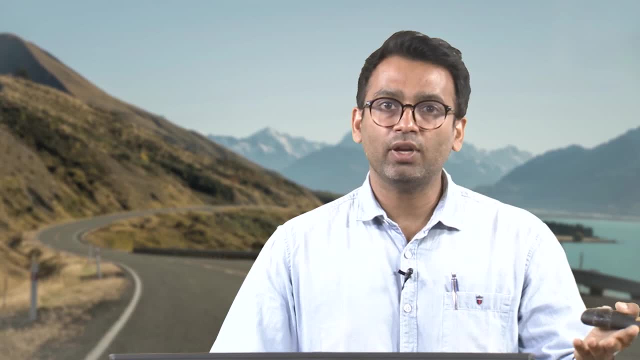 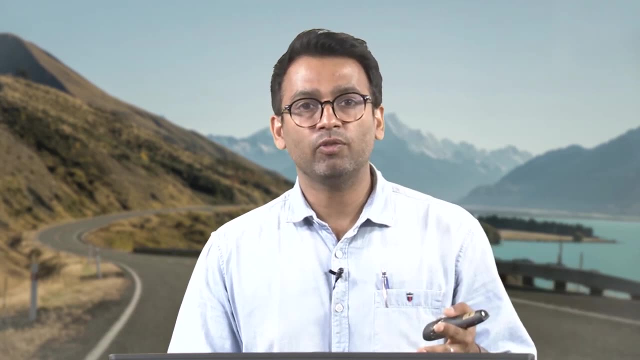 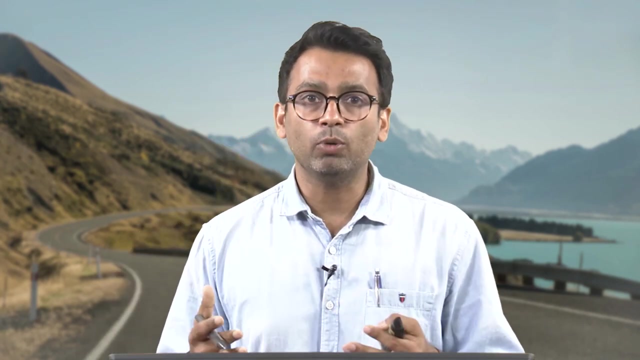 where we have some specific amount of traffic for which i am designing the pavement, where i have a specific number of years for which i am designing the pavement, and so on. so for pavement analysis and design also, we need to test these materials and obtain the inputs that are required during. 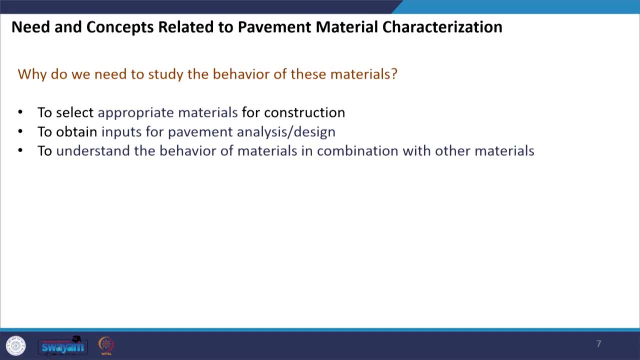 pavement analysis and then design, then we also need to study this material to understand the behavior of the materials in one hand and also the behavior of the materials in the other hand, also in combination with other materials, because my pavement is actually a system. even one layer, let us say if you are talking about a concrete mixture, if you are talking about a bituminous. 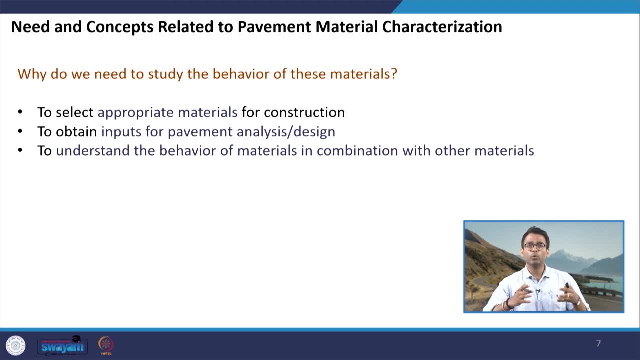 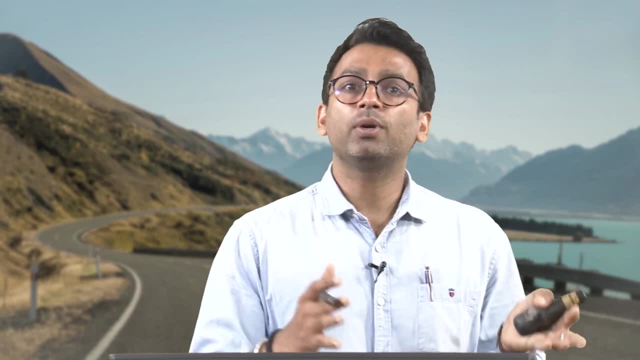 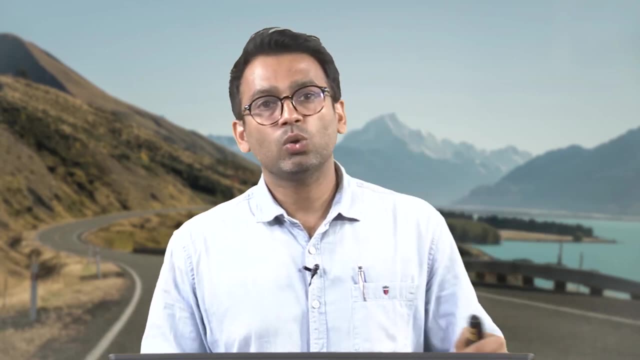 mixture, that is a system. when i say system, it is a composite of different materials. so sometimes i am also interested to know about the properties of this composite, correlating it with the properties of the individual components with which it is made. so this is also one of the reason that i 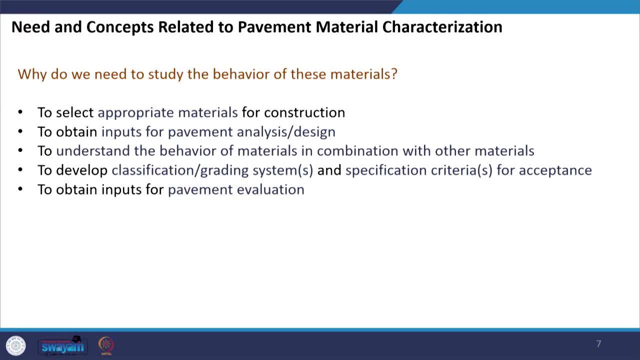 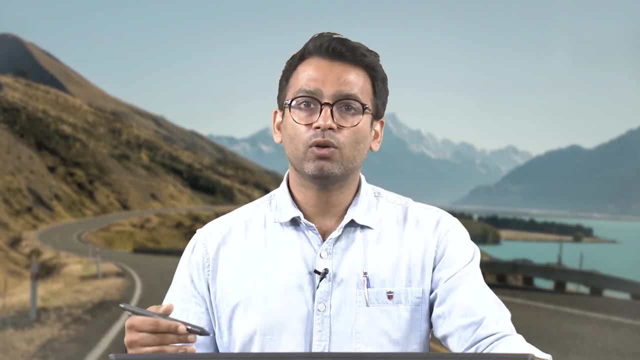 want to study the behavior of the materials in one hand and also in combination with other materials, of individual materials. the study of materials is also required to develop classification and grading systems. for example, in case of bitumen, we have v g ten viscosity grading system v g ten. 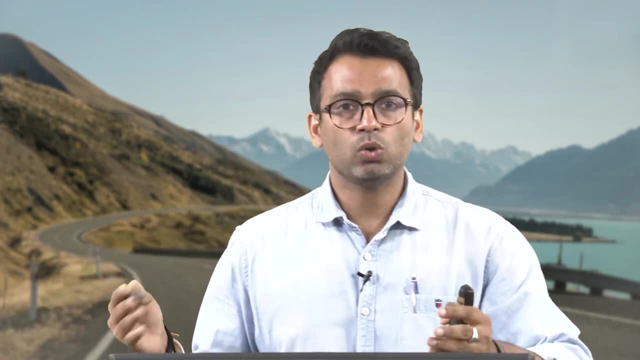 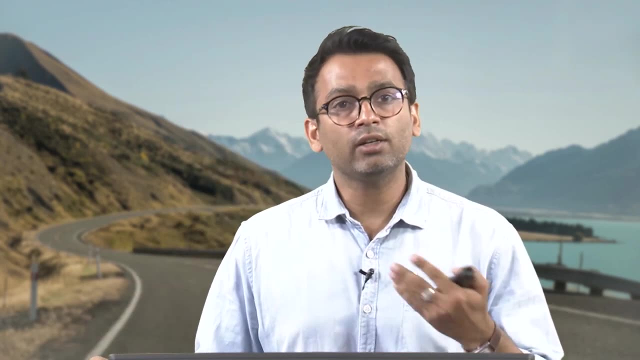 v, g, thirty, v, g, forty and so on, ah. similarly, if you talk about bitumen emulsions, we have different grades ah depending on the setting time of the emulsion. we have rapid setting emulsion, we have slow setting emulsions. so, in order to 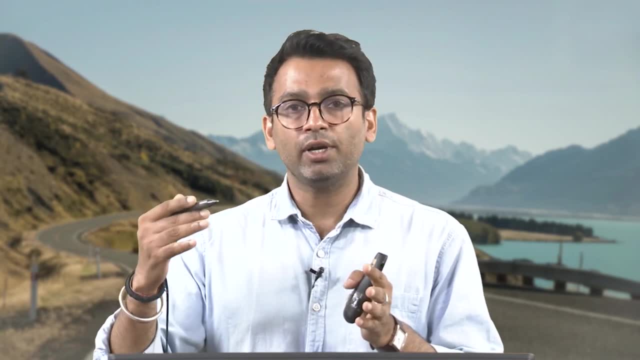 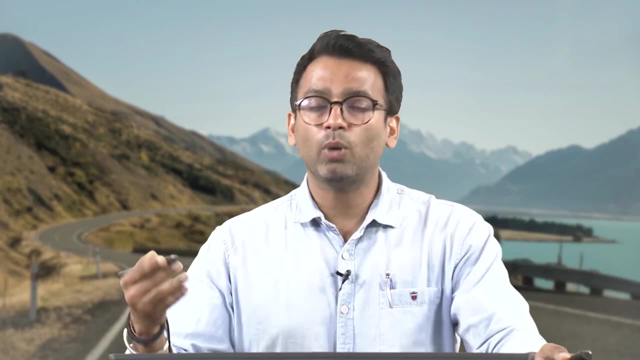 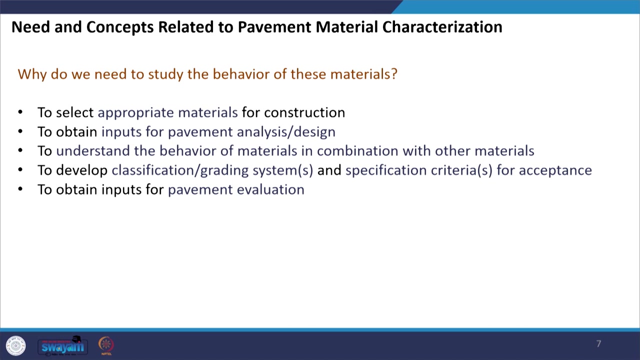 classify or grade the individual materials under different categories. we need to test this material. we need to study the properties or certain ah, different properties of these ah materials. further, the study of materials is also required to get inputs for pavement evaluation. now let us say you already have a constructed pavement. let us say that after. 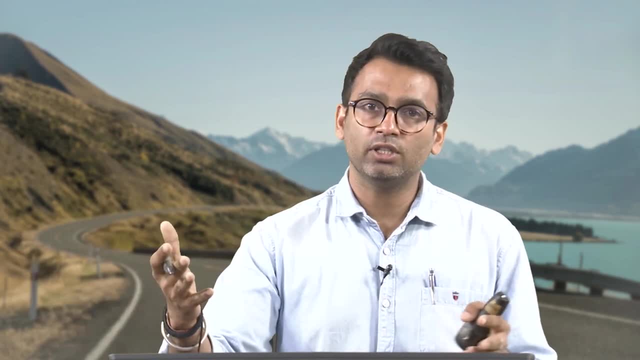 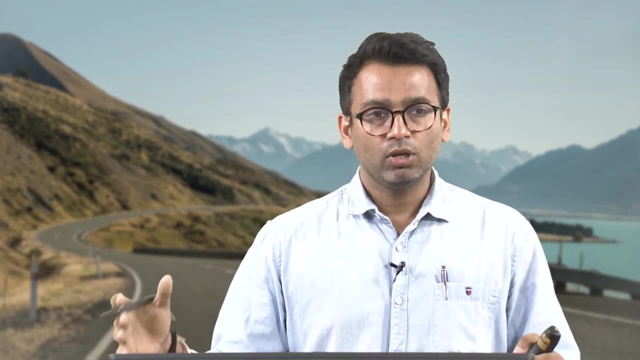 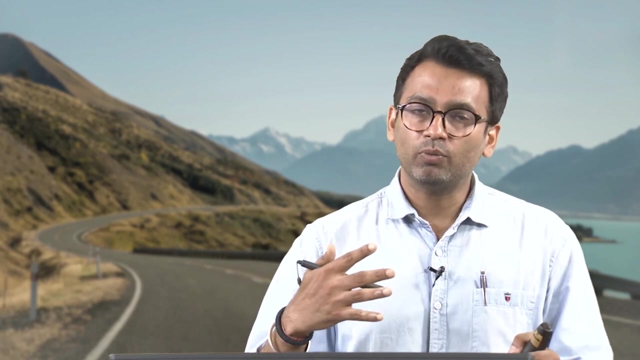 you have constructed the pavement for twenty years and after five years you visit the pavement and you want to know what is the remaining life in that pavement. so how will you know the remaining life? ah, one way is to cut open the pavement, get the materials, ah from the pavement, test it in. 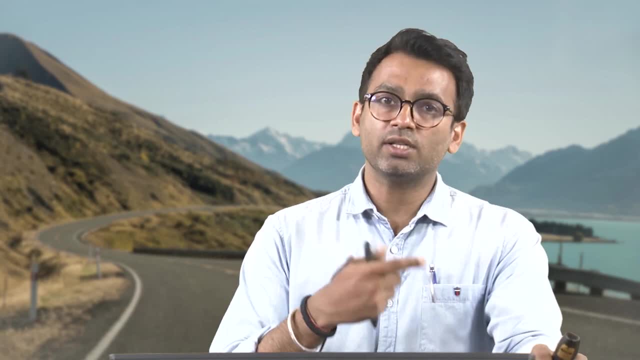 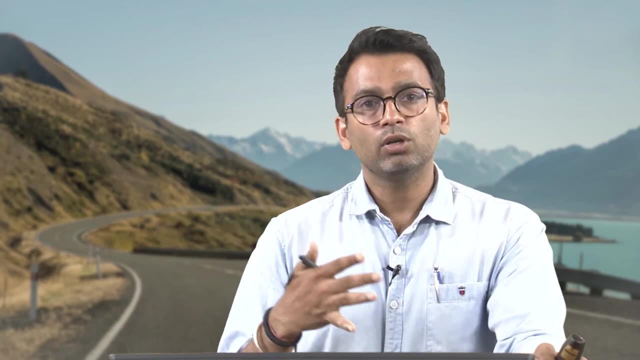 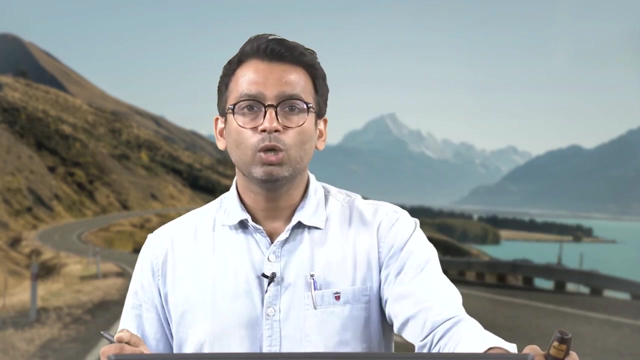 the laboratory try to see that what is the present property and then the property we used during pavement design. we will use a back calculation process to see that what is the remaining life of the pavement, using the same pavement design procedure. we adopt it while designing the pavement. 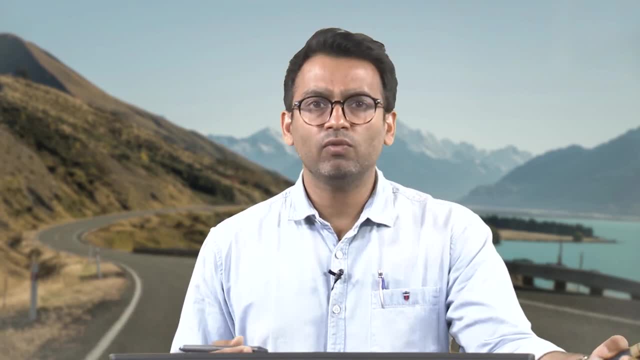 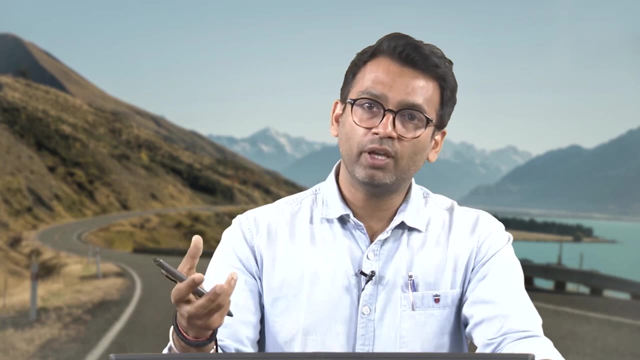 another method is to ah go for non destructive testing, which is the most common way of analyzing the pavement presently. we will take deflection sensors, we will give some load to the pavement, we will measure the deflection bowl, we will get the response, and this response we will 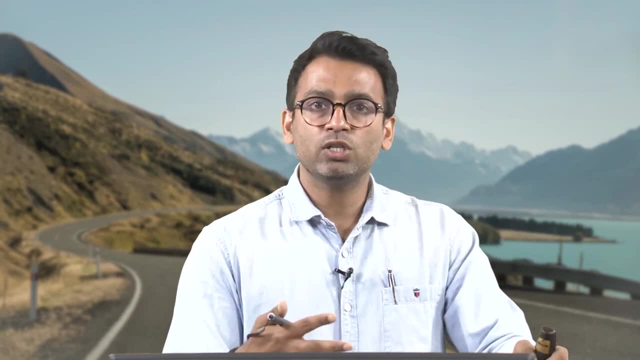 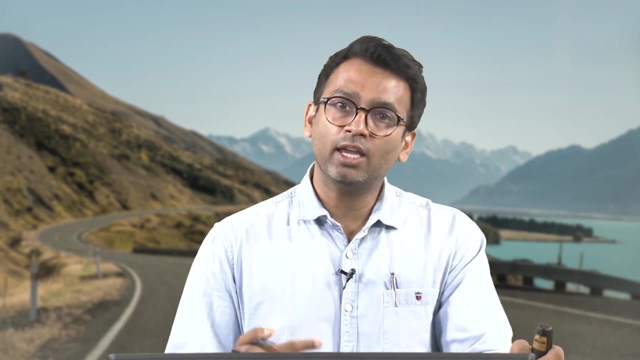 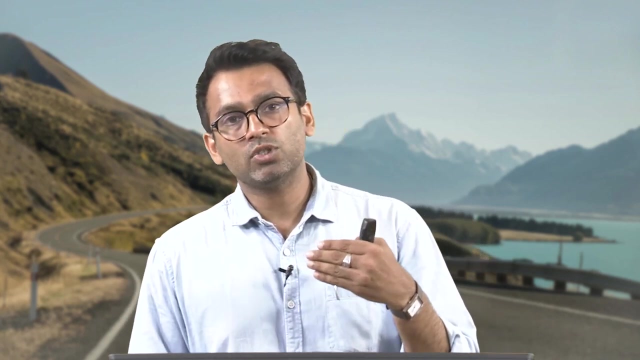 analyze, using some ah available methodologies, using some available theories, ah to back, calculate the properties of the existing pavement and these properties will again be put in the pavement design process to calculate the remaining life of the pavement. So ah study of these material is also required for pavement evaluation. 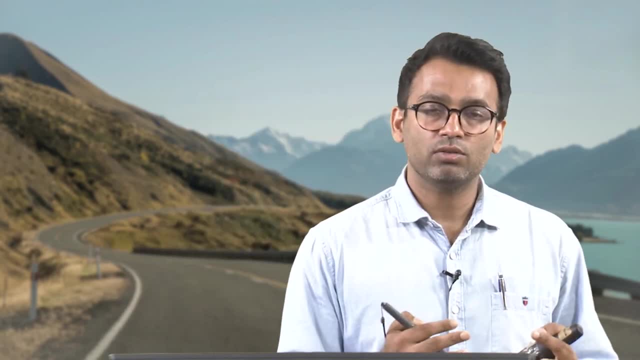 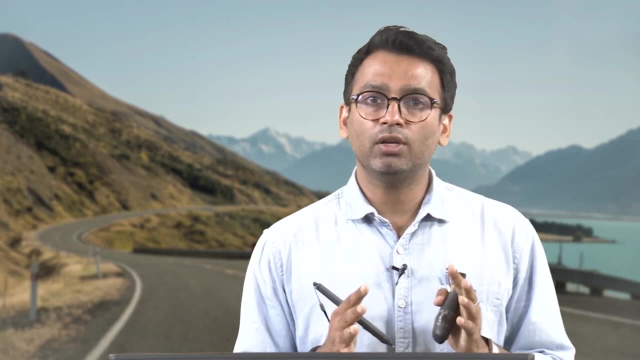 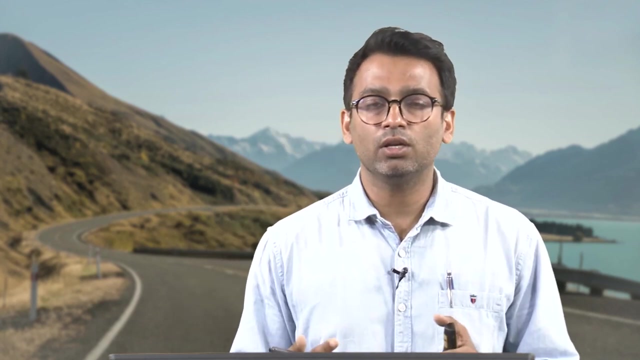 Now we have identified various important reasons. there can be other reasons also in the list, but these are some of the important reasons for which we need to study the behavior of these pavement materials. Now the question is: once we know that there is a need, then 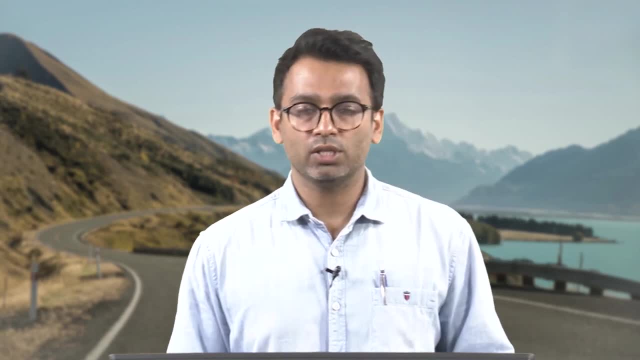 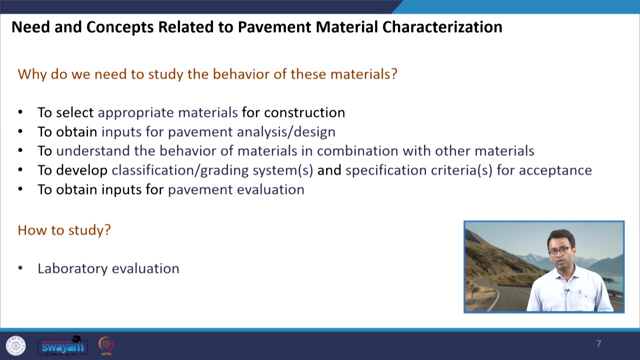 how are we going to study ah, you know, these ah properties, or ah, the desirable properties? The most common way to do it is to do a laboratory evaluation. you have the material with you, you know, you have some list of test available, some list of test developed as per specification. we will subject the material to those testing. 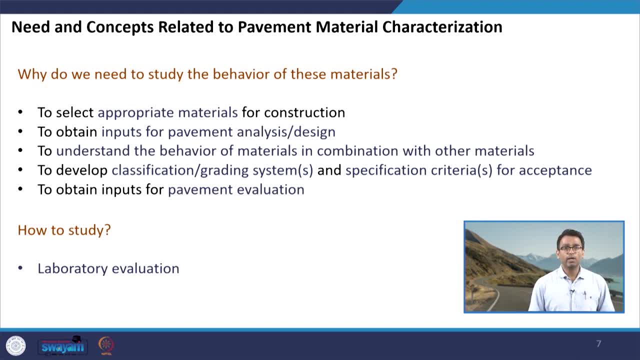 we will get the results and then we will ah be able to characterize this material. So one way is to do laboratory evaluation. We can also do field evaluation, as I just mentioned that if we are interested to know the ah material properties of some existing pavement system, then we can do some non-destructive 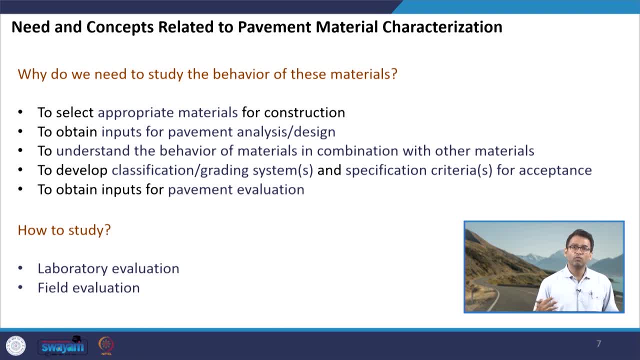 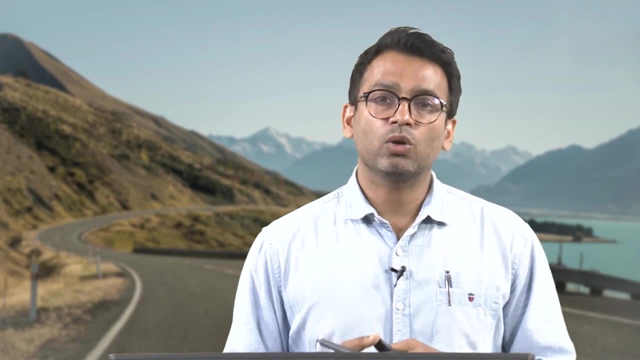 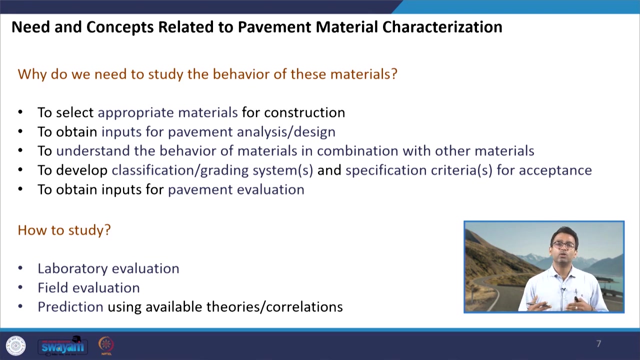 testing. using the results of the non-destructive testing, we can back calculate the material properties. If we are not in a position to do, you know, both these type of ah ah evaluation, then we can also use existing theories or correlations to predict зм the properties. when i say existing theories it means ah, let us say you are interested. 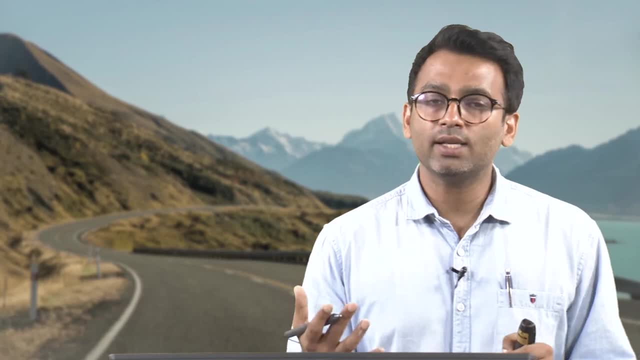 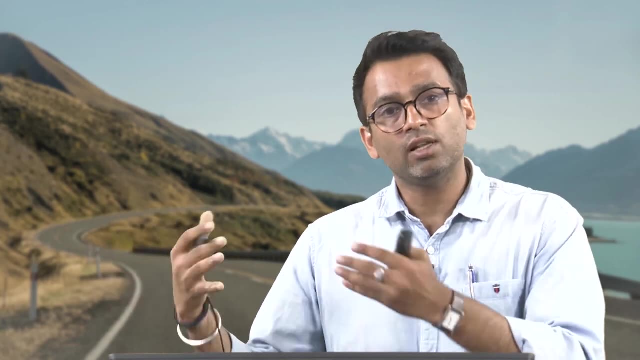 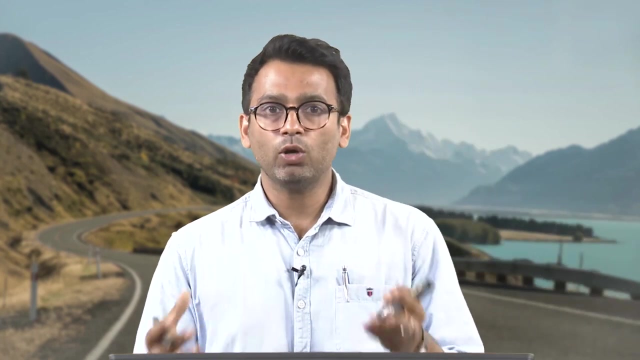 to know the resilient modulus of a bituminous mixture. now, to know the resilient modulus of the bituminous mixture, you have to subject the mix to a specific testing procedure in an equipment which itself is very costly, the operation of which is very complicated. ah, therefore, ah and, but somehow you want to know the property. so what you will do, we will search. 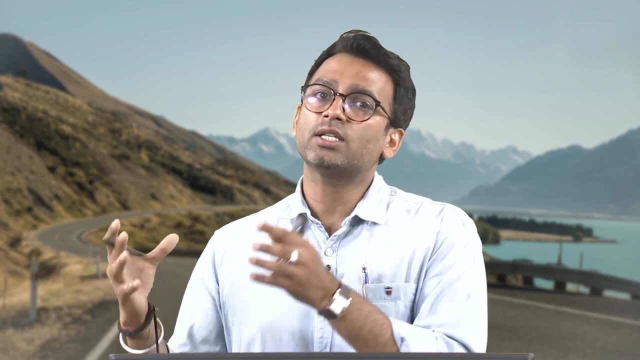 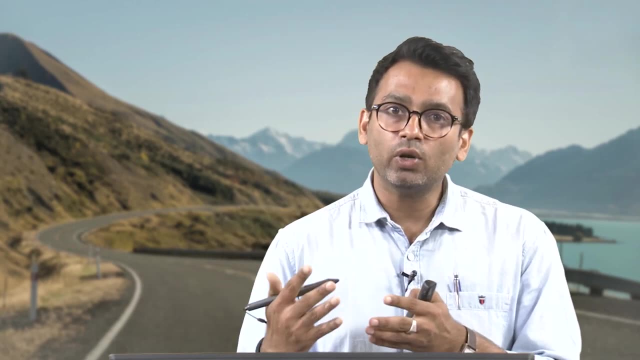 for alternate methods. maybe i will do some simple testing on the bituminous mixture using a method which is available, ah with me, and then i will try to see if there is a correlation between this test, which the simple test which i am going to do, and the resilient modulus. 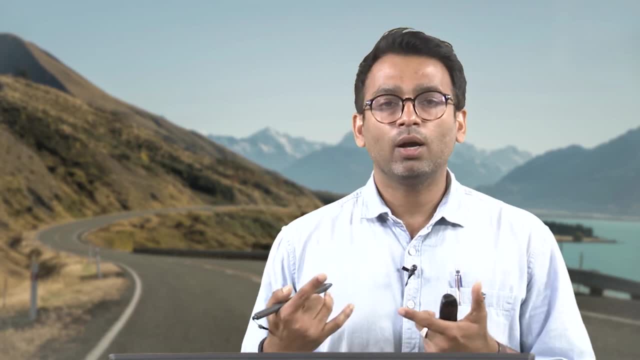 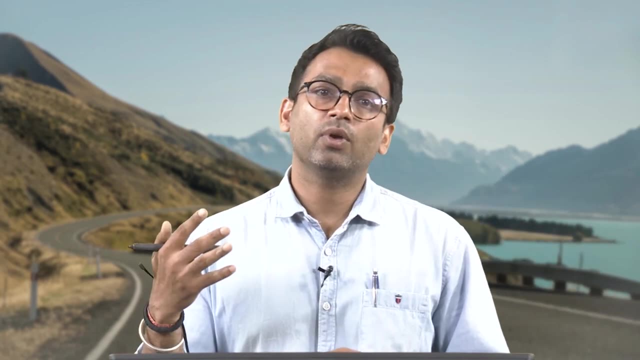 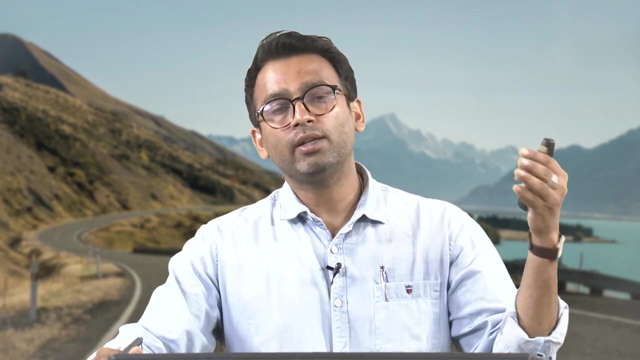 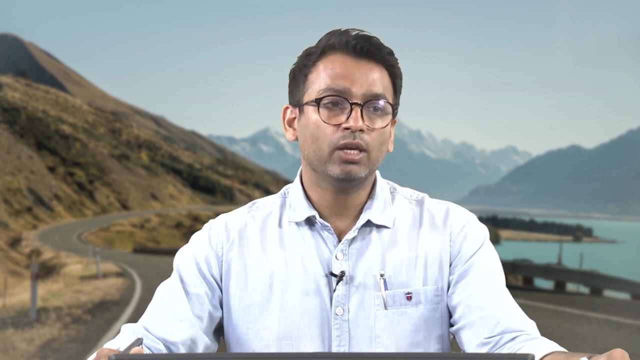 which i desire to find out or i desire to ah evaluate. all right, so using the existing correlations and theories, we can also predict ah various material properties. it is very important for us that before we adopt any testing procedure to characterize the material, we should be very confident about the robustness of that particular equipment, so that the property 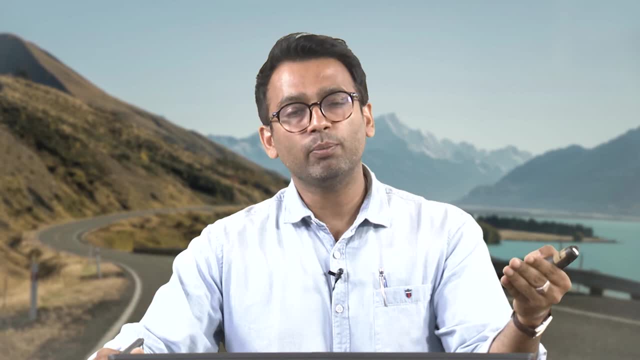 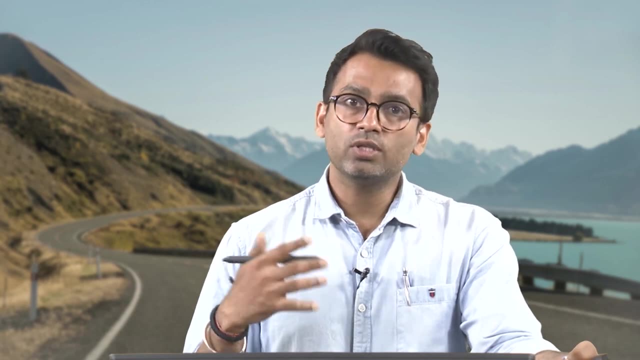 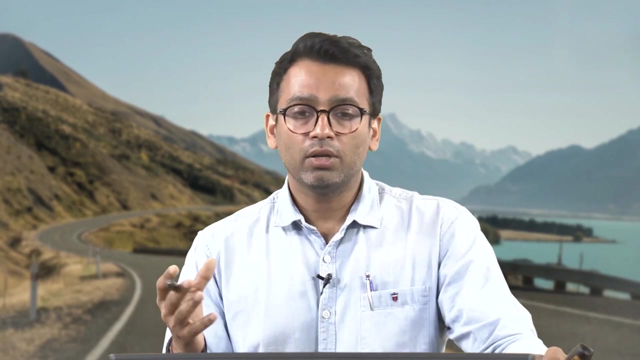 which i am getting from that, from. you know, subjecting the material to that particular testing should be able to ah guide us to use that material for the specific project. when i say specific project, try to imagine it in this way that there can be, you know, the same material can be used. 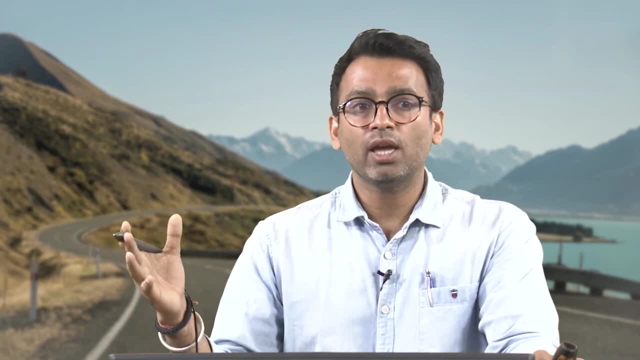 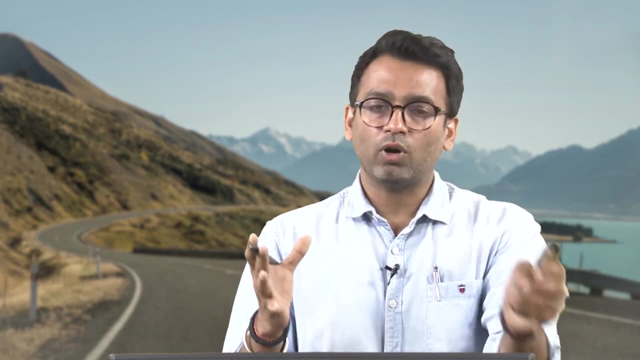 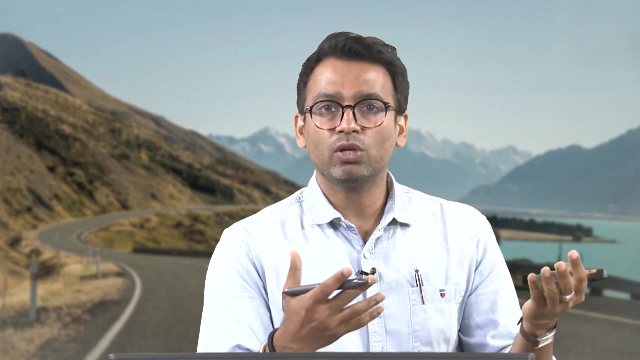 in various different projects, and various different projects have their own objectives, have their own requirements. maybe you are using one time ah in one project. you are using this material in a location which is subjected to, let us say, very high temperature. the temperature of the environment is very high. the same material you are using in some other location where 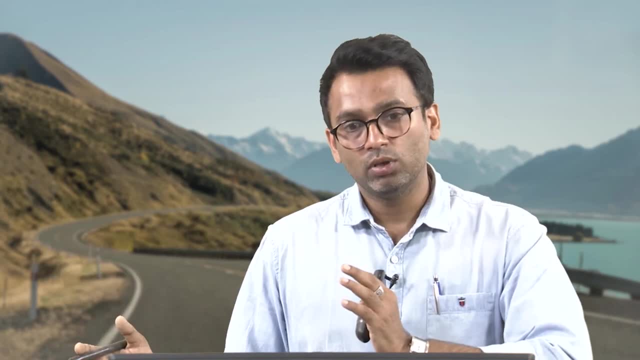 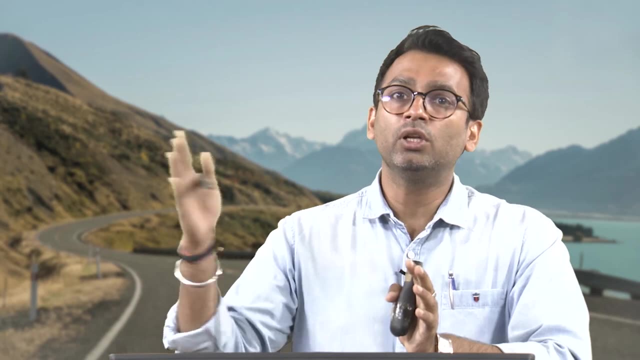 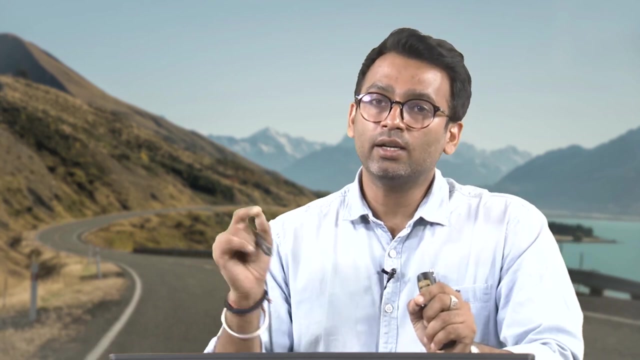 the temperature of the location is very low. Now if the response of this material is temperature dependent, then the material will behave differently in both the locations subjected to same loading conditions. Therefore, in the laboratory I cannot use a single test to characterize this material for both the locations, which means the experimentation. 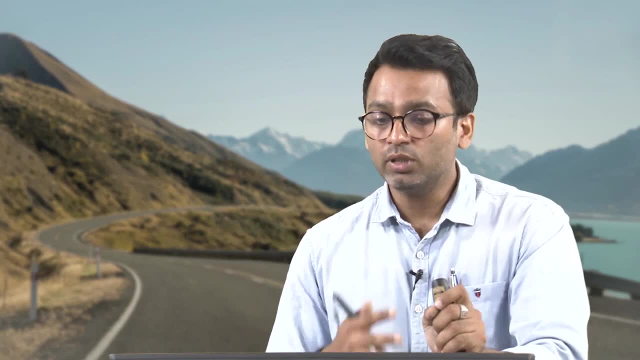 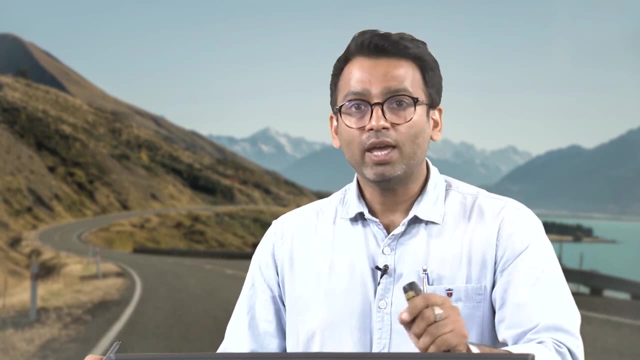 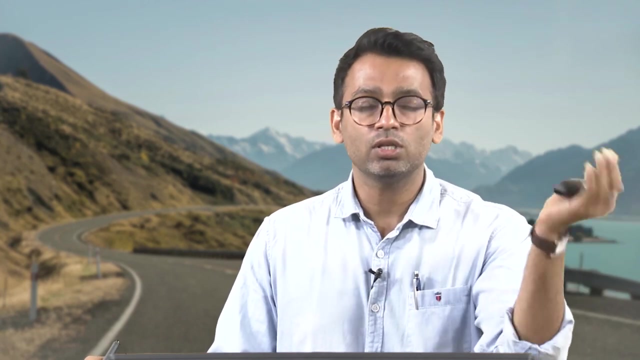 itself, which I am choosing, should be project specific. Now, this is very important, but not necessarily it is always considered as per the available specification. but we have to think about it, we need to ask questions regarding the existing specifications, regarding the existing methodologies, and we have to ah see or we have to explore that. which are those? 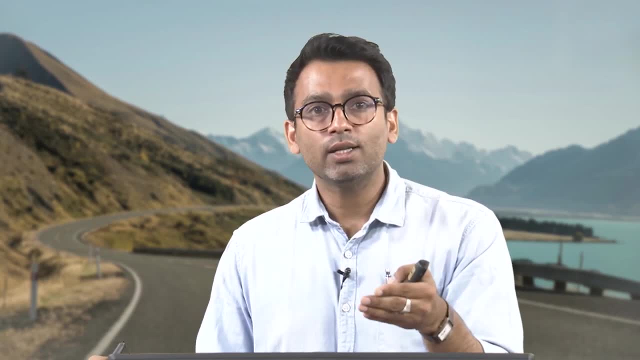 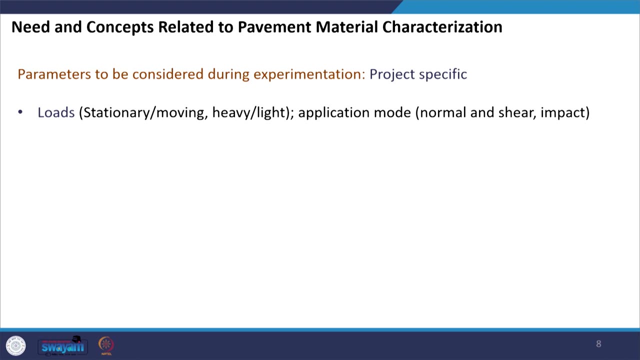 test methods which are really useful to understand the behavior of the material for the purpose for which I am using it. So, ah, some of the critical parameters which I have to ah consider before doing the experimentation is loads. Load is one of the very important. 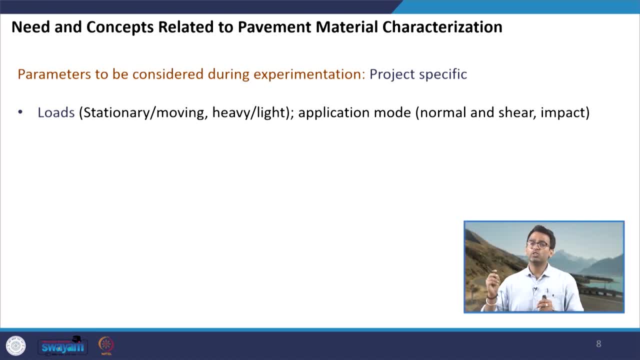 parameter. So I have to understand that the material which I am going to use will be subjected to, or the material which I am going to use in the pavement system. So that pavement system will be subjected to which type of load will it be subjected to? stationary load? 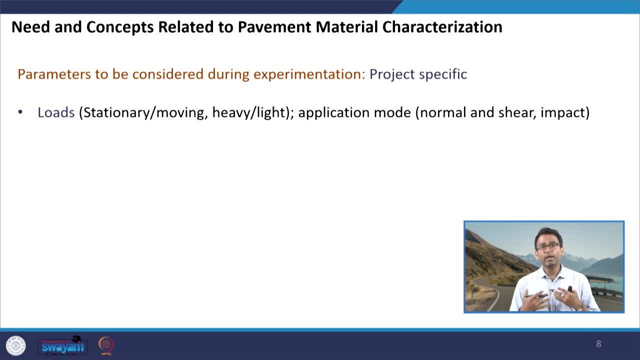 will it be subjected to moving load? what will be the magnitude of the load? will the load subject very, or will the load impose very high stresses on the pavement? So I have to see the layers and the materials. will the load ah be, ah, you know, not very high it? 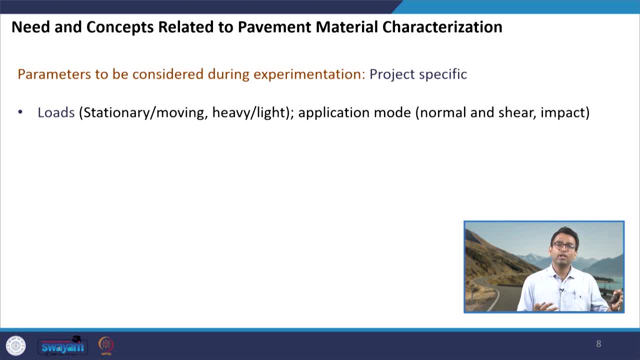 will it be light and accordingly, in the laboratory I have to see the response. Say, the load is moving and the material which I am ah going to use is very susceptible to change in you know frequency, or the ah, frequency of the loading, or ah. you know the magnet magnitude? 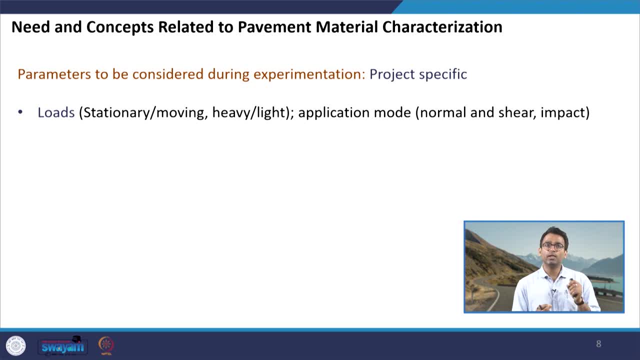 of the load. let us say, And I am using a stationary test- ah test- to get some material property. So this material property which I get using the stationary load may not tell me the or may not tell me about the exact, exact response or exact way. 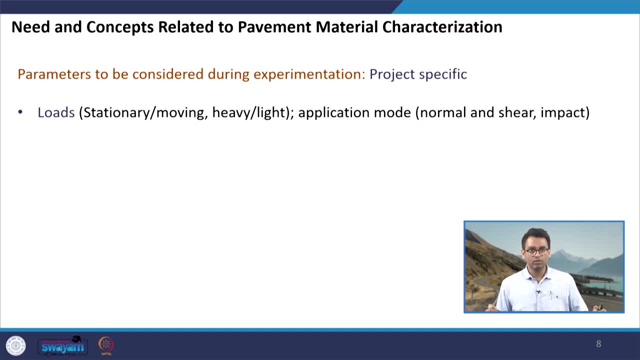 this material is going to behave when it is actually used in the field. So if there is a moving load and my material is susceptible, or the response of the material is, ah, dependent on the- you know- frequency of loading, then it is better to test ah the 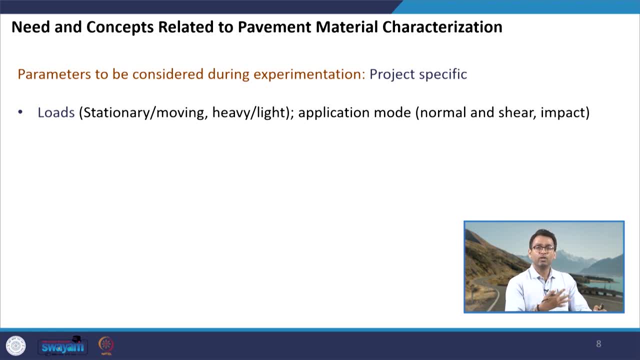 material, ah Meaning. you know similar ah level of frequency at which we are anticipating. you know the material will be subjected to in the field. Similarly, the x, the magnitude of the load. if the load is going to be very heavy, I should be able to apply higher stresses in the laboratory. 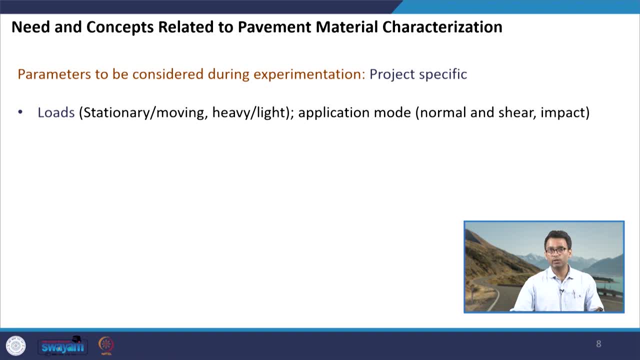 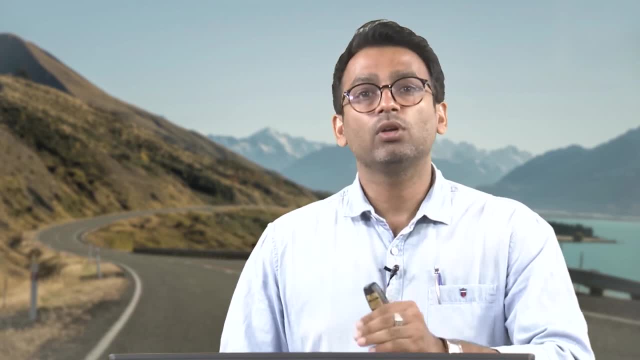 to see how the material will respond to that particular magnitude of stress. Then, ah, when we talk about load, we also have to see the application mode. are we studying the tensile properties? Are we studying the compressive property of the material? are we studying the compressive? 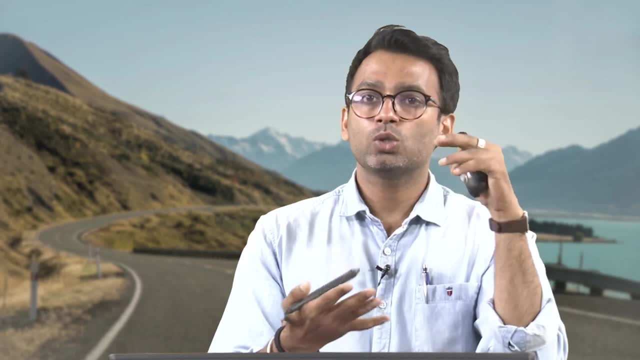 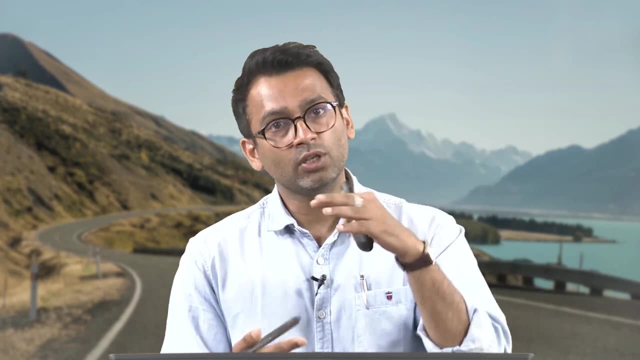 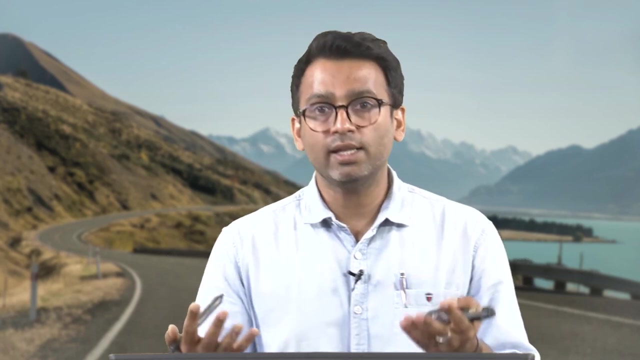 property of the material. are we studying the material under shear? So all these different- you know- modes of loading will change the response. some material are very good in compression but very weak in tension. some materials have high shear strength but may have lower compressive strength or lower tensile strength. So we have to understand that this material 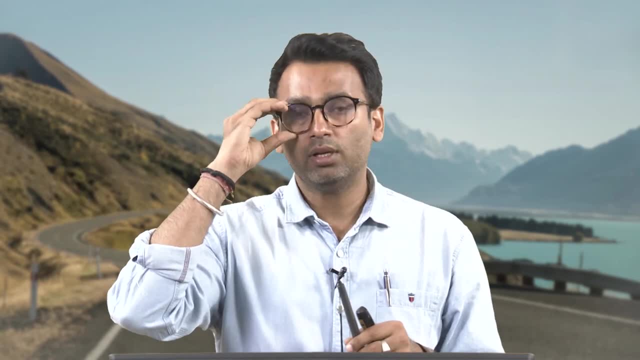 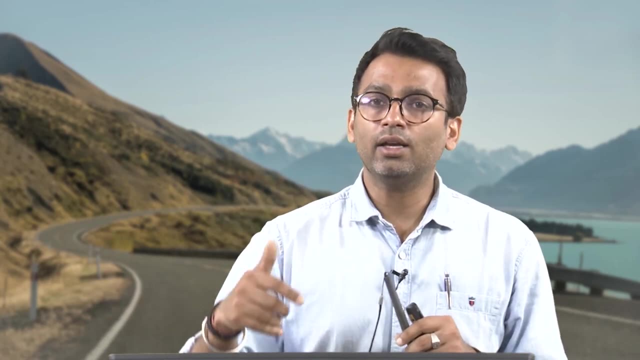 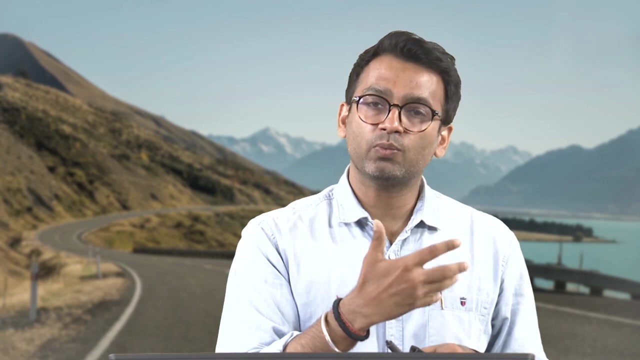 or this ah mixture which I am going to use for pavement construction. What mode of load this loading will that be subjected to in the actual field condition? If I know that the critical mode to which it will be subjected is shear, then I have to test ah. I have to find out the property or the response of the material in the laboratory. 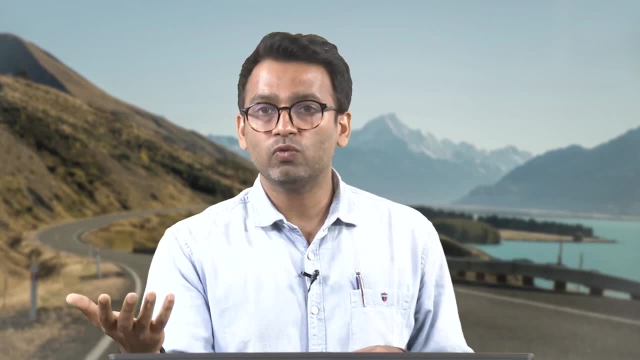 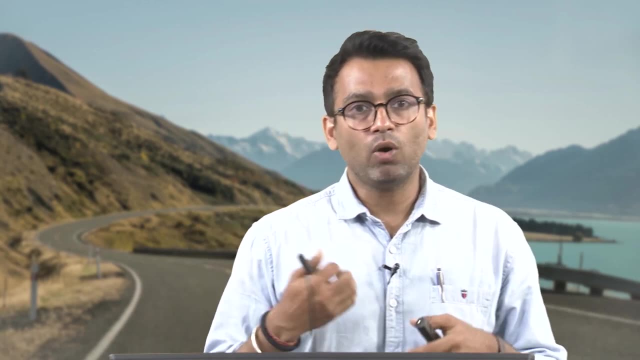 using a shear loading. If the critical load, which is which will be applied, which will lead to the failure of the specimen, is a compressive load, I need to test the material in the compressive mode. So, accordingly, we have to think and we have to adopt those testings which will 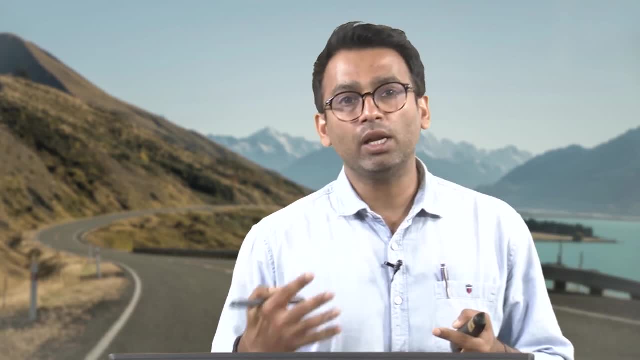 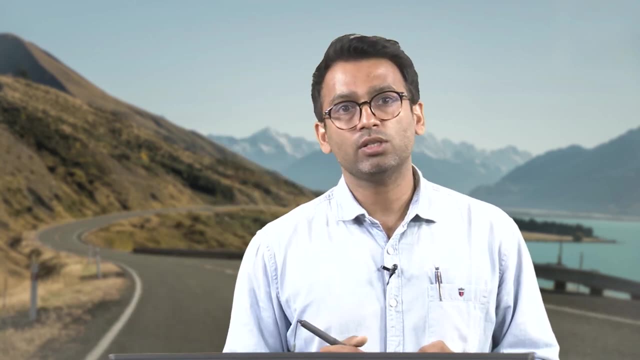 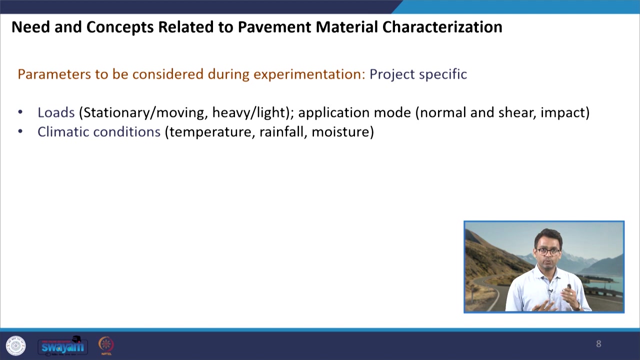 give me realistic property of the material corresponding to the project at which I am targeting. We also have to look at the climatic conditions. climatic conditions ah mainly include the influence of temperature. for example, ah bituminous material. they are viscoelastic in nature. So, as I just mentioned that, if you heat bitumen 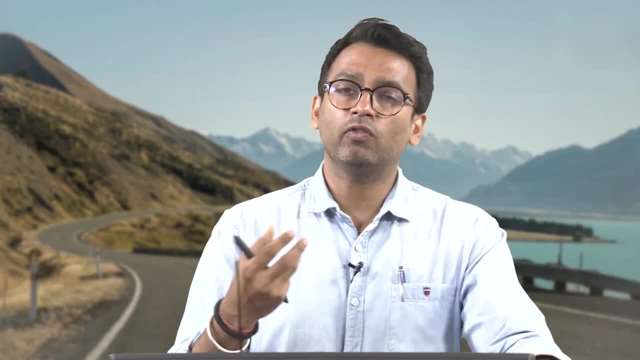 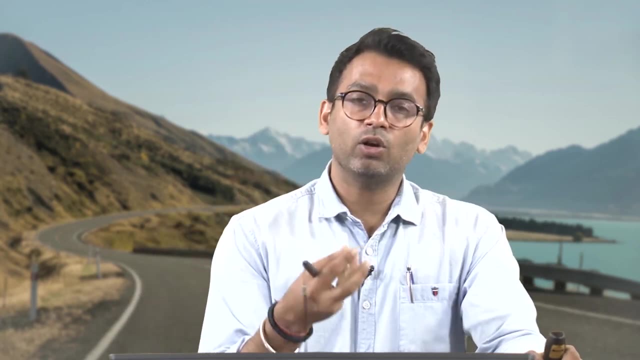 it will become fluid. if you ah reduce the temperature, it will ah solidify, it will behave as elastic material. So we have to see that the the material or, for example, if- if you take the example of bitumen, we have to see what is the range of temperature at which it will be exposed in. 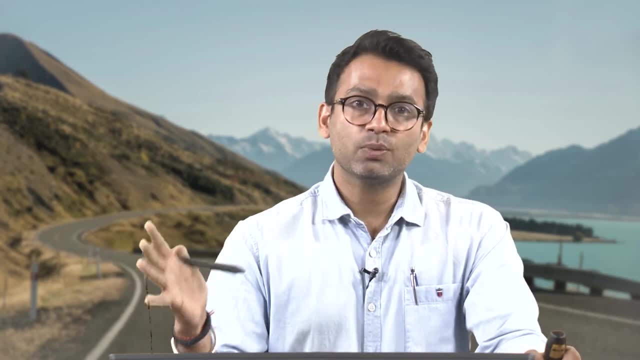 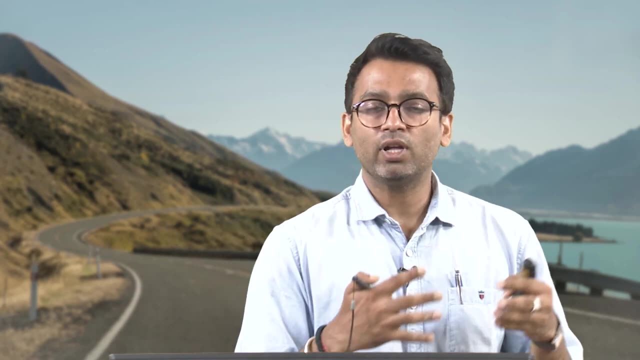 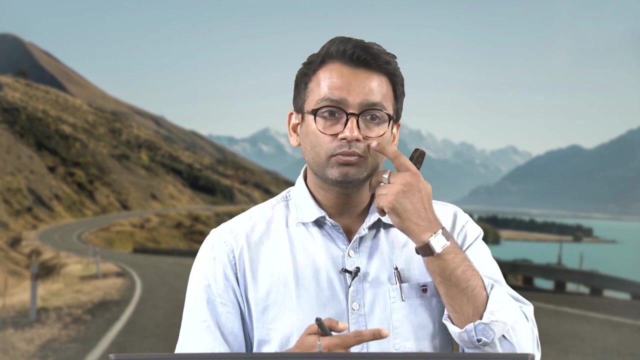 my project And accordingly I have to know the response of the material under that varying degree of temperature in the laboratory. And then you know, once I have ah the ah response of the material and I am confident that this material will behave ah desirably, then I will. 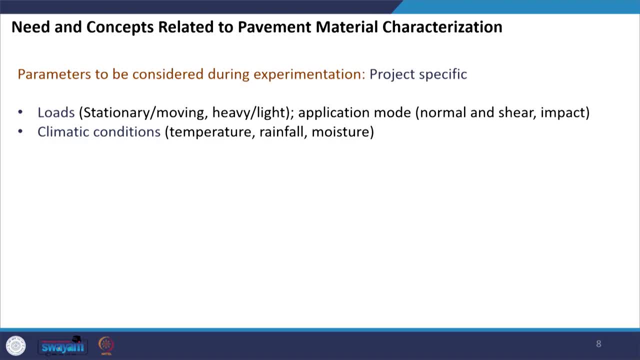 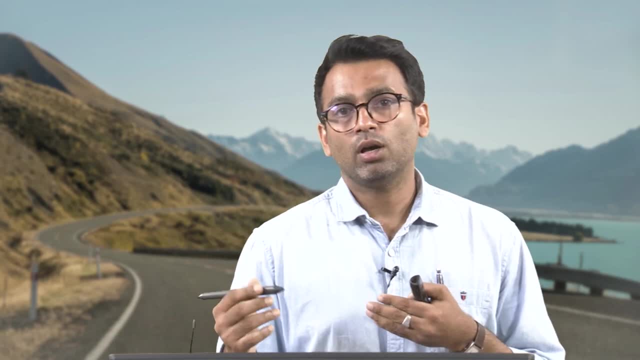 be able to use it in pavement construction. We also have to see the effect of ah, rainfall or moisture. you can say, for example, you take soil, ah. we will discuss that. the properties of soil is highly dependent on the change in moisture content. So there is one particular. 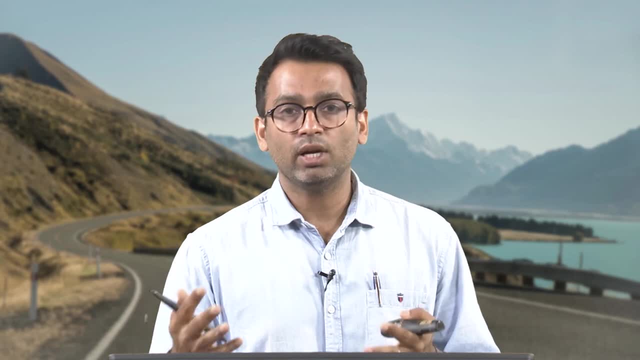 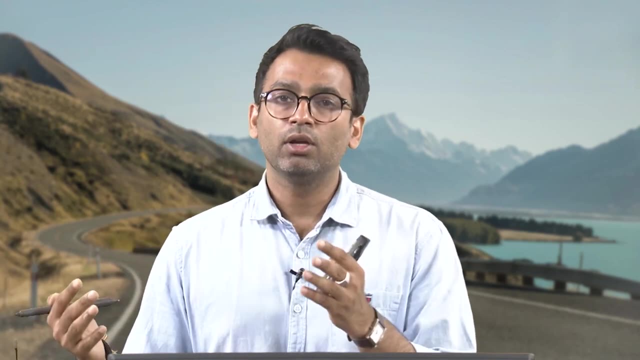 moisture content at which the soil has the highest density. that is the optimum moisture content, but maybe during monsoons my- ah, my soil, or the subgrade, gets saturated and the moisture content changes, Which means my pavement will become weak. So I have to see that: what is the moisture? 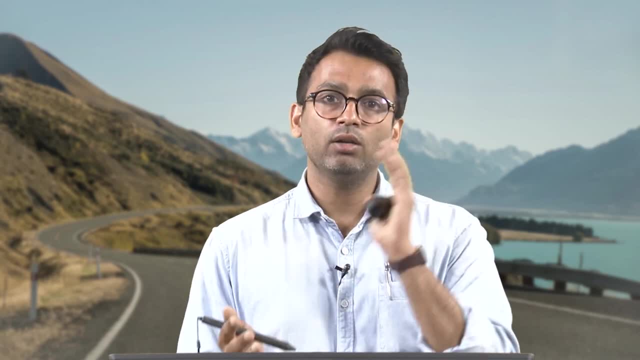 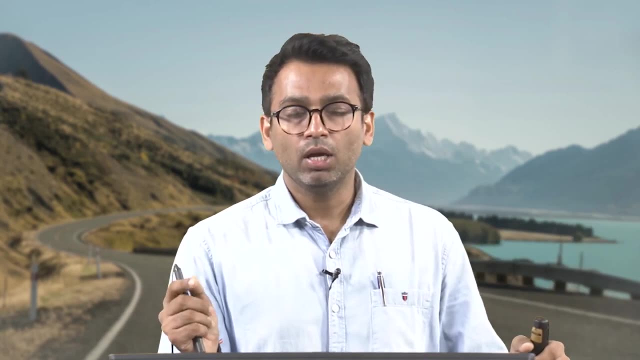 content at which I should expose my soil for testing in the laboratory, And the same in response which I get should be used during the pavement design. If we have a location where we are anticipating that the moisture level is not going to change, then using a 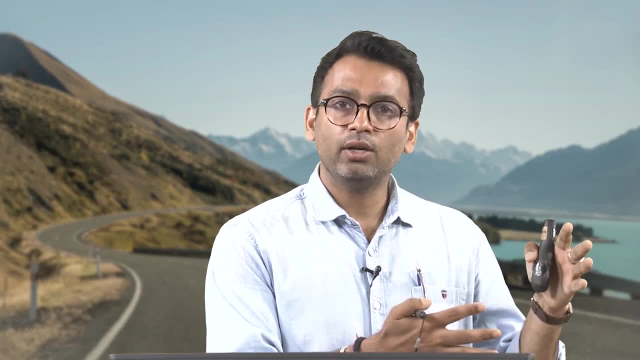 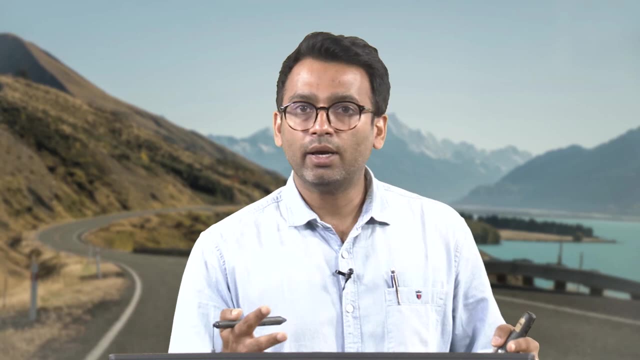 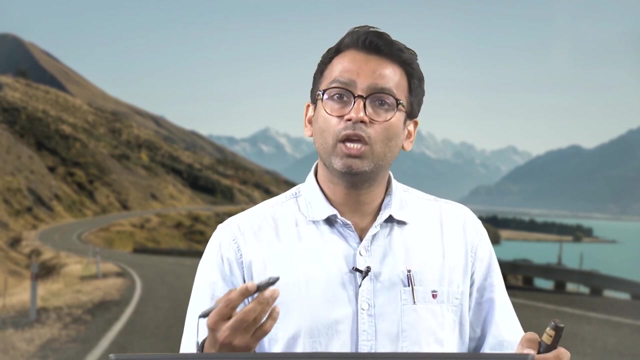 very ah. you know high moisture content or you know ah subjected or ah. subjecting our sample to So higher degree of moisture may not be correct because that will not lead to an economical design. If I know that the material is not subjected to ah, change in moisture content. 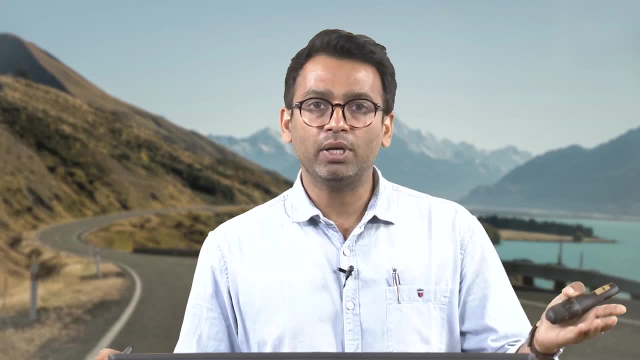 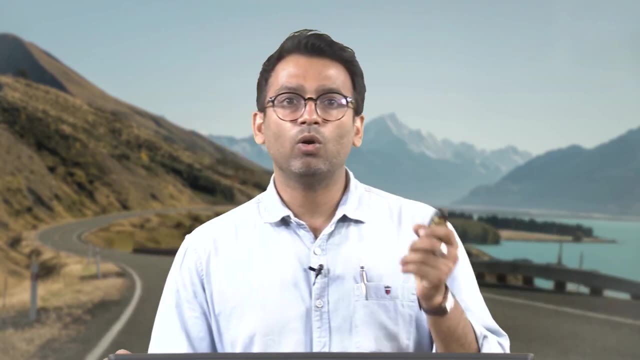 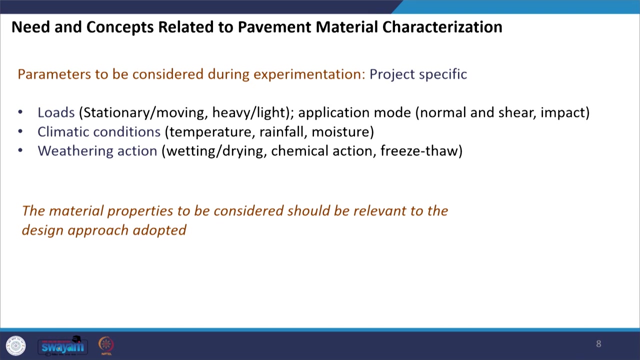 then I should use ah, the corresponding desirable property, and we need not see the behavior of the material under worst conditions. So you have, we have to decide again all this parameter based on the specific project and the location. Then we also have to see whether we are using the materials in a location where they have. 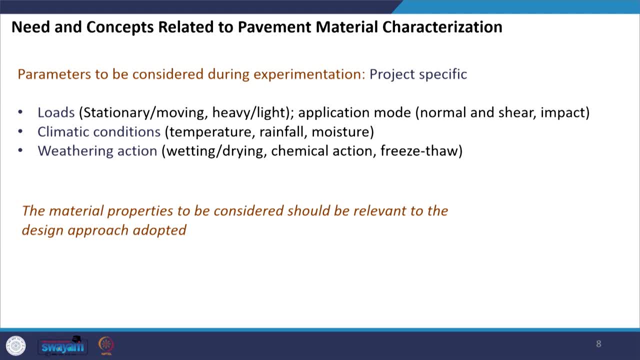 there are cycles of wetting and drying, where there there can be chemical action, where there can be cycles of freezing and thawing, and accordingly i should also test the material in the laboratory because you know the the response, the behavior of the entire pavement structure can change ah depending on these ah parameters and these criterias. 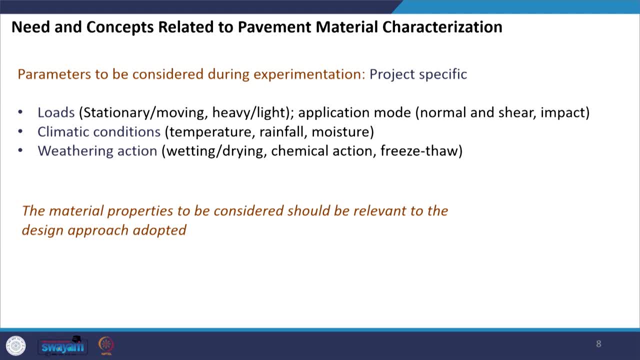 so the material properties to be considered should be relevant to the design approach adopted, as i mentioned. for example, in the design approach, if i am a flexural strength is an input, i should do the flexural strength testing. if resilient modelers is an input, i should be able to find out the resilient modelers. so, depending on the pavement design, 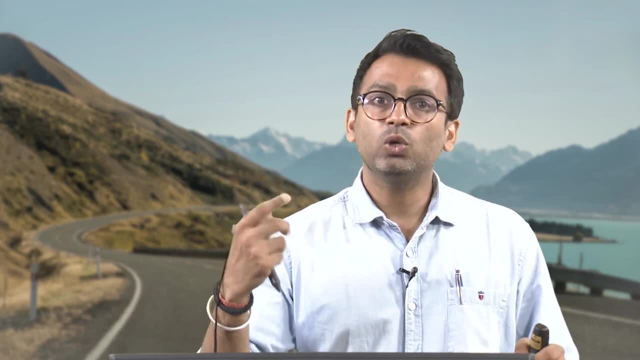 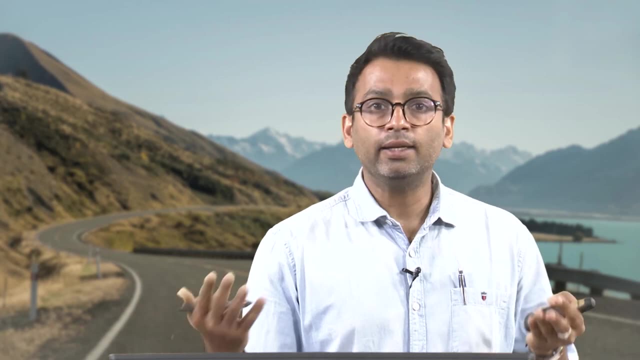 i should take the appropriate test, For example ah. in US, when doing the pavement design, they take the dynamic modulus of the ah bituminous layer as an input, while in India we use resilient modulus. So why should i do a dynamic modulus test in the laboratory when resilient modulus is? 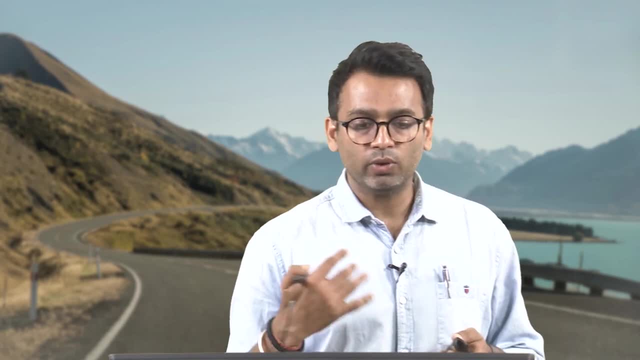 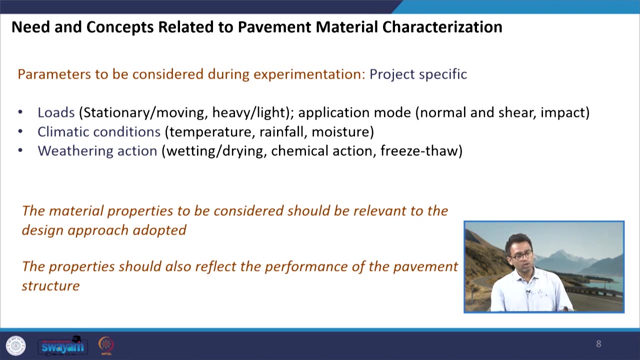 this an input in the pavement design. So this is, you know what I am trying to explain: that the material properties to be considered should be relevant to the design approach adopted And these properties, of course, should also reflect the pavement performance. When I say 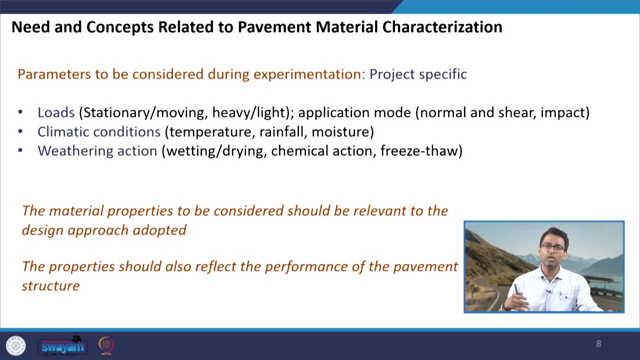 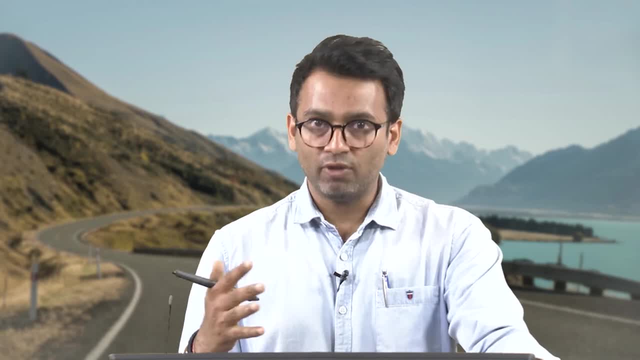 the performance of the pavement structure. I am mostly indicating about the critical failure mode, the type of distresses which is occurring If it is a flexible pavement, if you have fatigue cracking, I should know that. what are the parameters or what are the 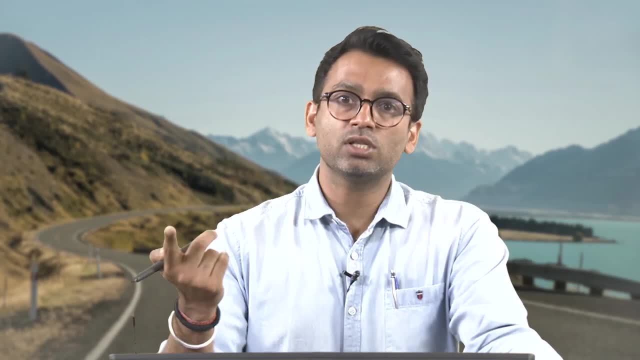 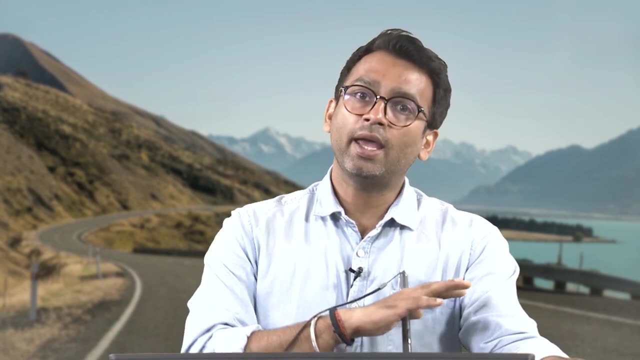 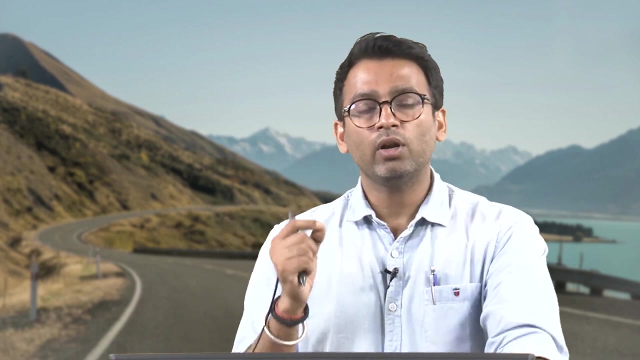 properties of different layers that can be related to this, ah fatigue cracking, And accordingly those parameters I should be testing in the laboratory Instead of you doing n number of test which gives me no idea about the, you know, occurrence of fatigue cracking in the laboratory. So our target properties should also be chosen such that these properties 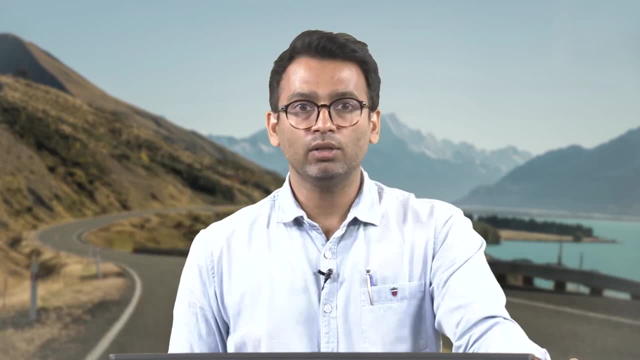 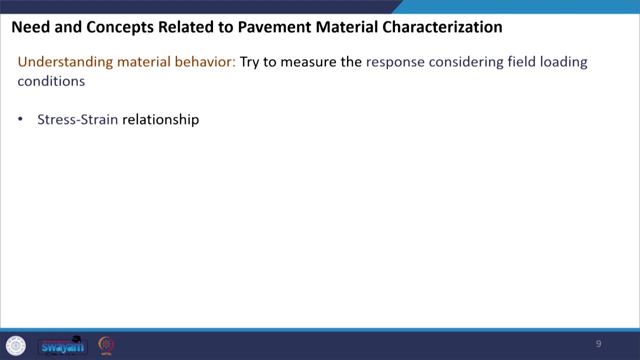 are related to the ah critical distresses that occur in the field, As I have been mentioning continuously that we have been mentioning continuously that we have been mentioning continuously that we have to measure the response, considering the field loading conditions, And the responses can be ah seen in various different ways. For example, I can plot a stress strain relationship. 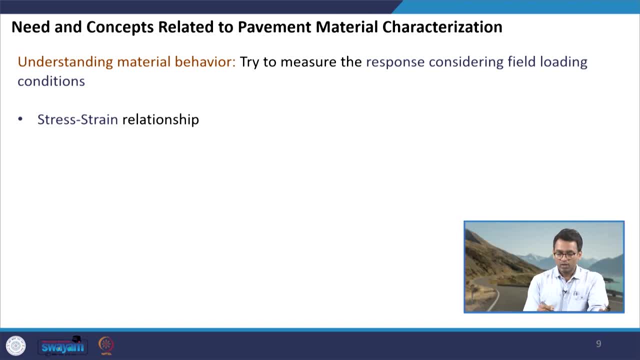 ah while doing the testing of the material. So that will ah. for example, if I am looking at the elastic modulus, then ah, the, the stress strain property, will give me the modulus. Now this can be linear, sometimes it can be non-linear, depending on the type of material. 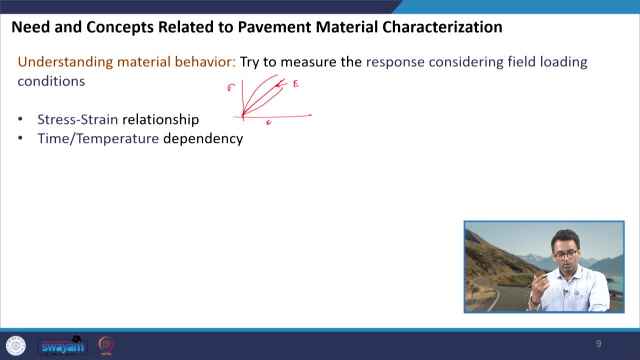 ah we are talking about. We are also have to see time and temperature dependency, specifically for those materials whose response change ah considerably with change in the time of loading or the temperature of loading. When I say time of loading here I am indicating the movement of the vehicles. 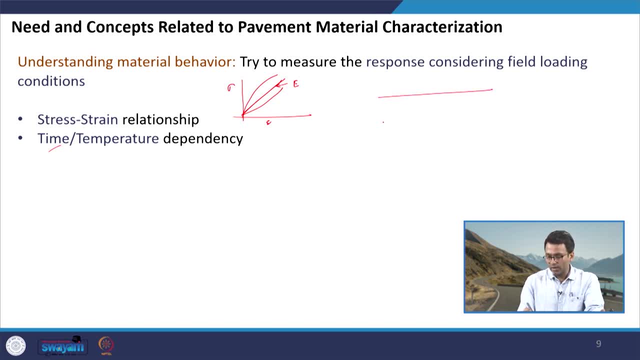 or speed of different vehicles. So, ah, in fact, in a pavement structure, you see that when a load ah moves, there is a deflection bowl which is created, there is a deflection bowl, There is a stress bowl which is created, and then ah materials in different layers. 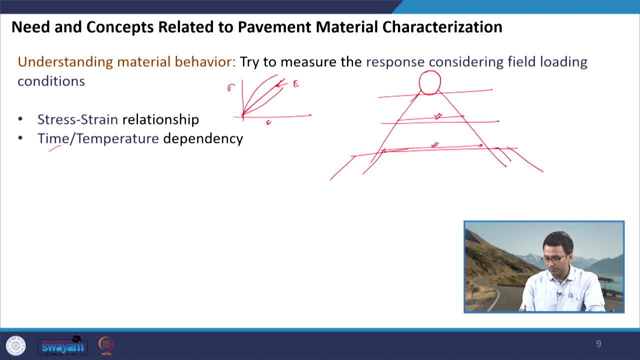 are subjected to different loading times. So if, if this is the length of tire imprint at the surface, then this material here is subjected to a you know ah loading ah period of L, if L, L is the tire imprint, While material in this ah particular location is subjected to a ah a time period of L dashed. 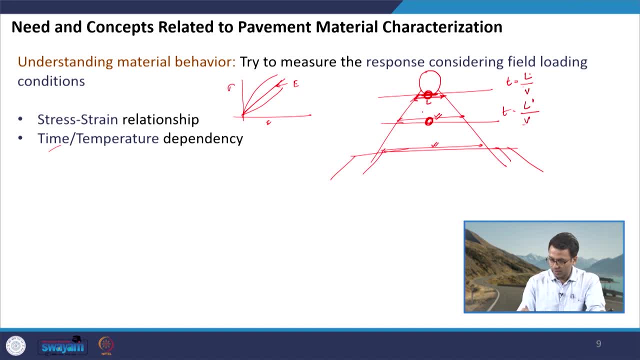 forth dash. if this is L dash, material placed here is subjected to a time period of ah L double dash. So you see, as you move down the ah duration of loading, it increases but the magnitude of load will decrease because the higher, highest magnitude will be at the surface. 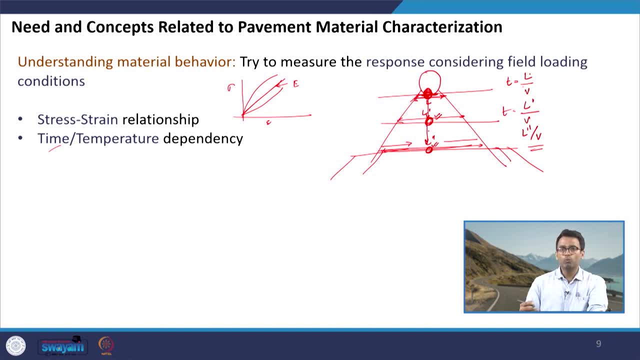 and then the magnitude will decrease as we go beneath. So both the. so when I am, you know, testing this material to get the response of this material, then the question is: in the laboratory, if I am doing a testing in which I can vary the magnitude of the load as well as the loading period, what loading period I should use? 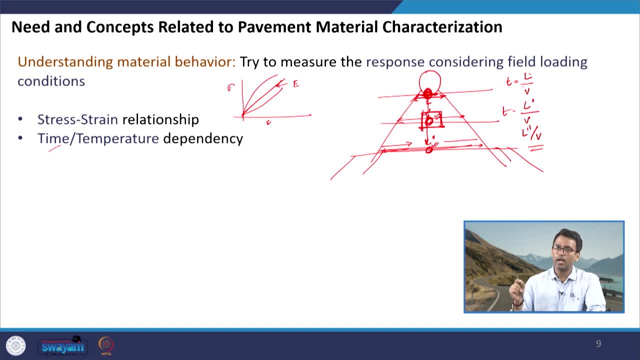 what magnitude of load I should use. And this magnitude of load and the magnitude of loading period, should you know replicate the standard conditions in the field, should tell me about the behavior of the material when it is placed in the field. Similarly, when I am testing, 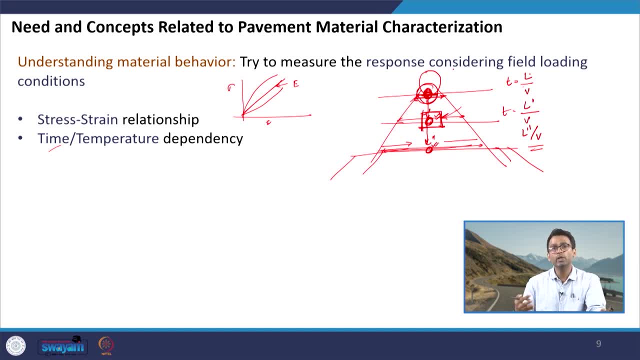 a material here I have to give a small, smaller loading time because the loading time is small here in the field but the magnitude of the load is high. So I have to select the stress levels, the strain levels, the ah loading period when I am testing material from this location accordingly, and you know, 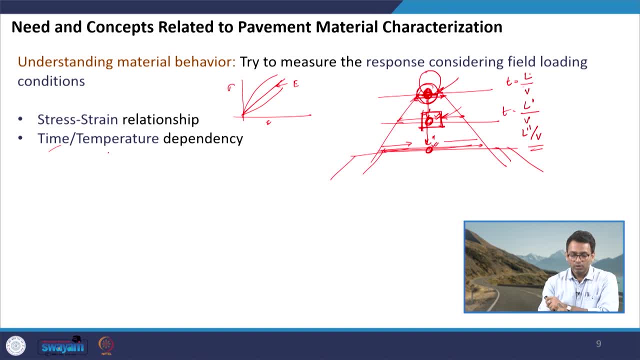 similarly for different layers. Talking about temperature dependency, I have to see ah that. if ah that, what is how the property of the material changes with temperature? Let us say I am talking about a bituminous mix. I might be interested that how the resilient modulus ah changes with temperature and then 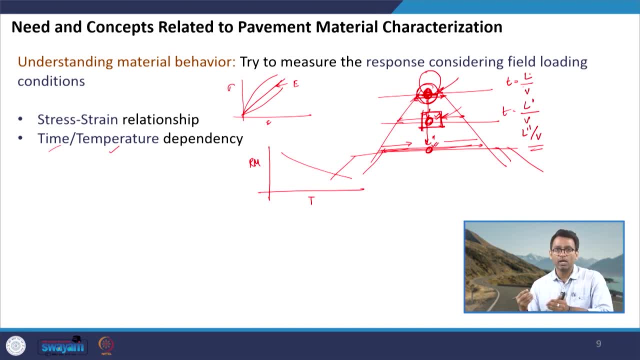 there is a particular standard temperature at which I am doing the pavement design. So I am more interested to find out the resilient modulus at that particular temperature. But if I am targeting for the properties at a range of temperature, I also have to see the 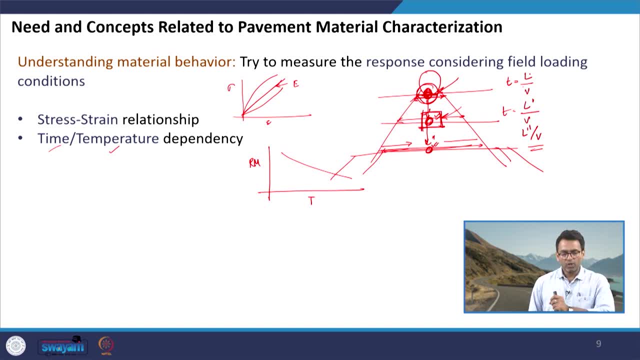 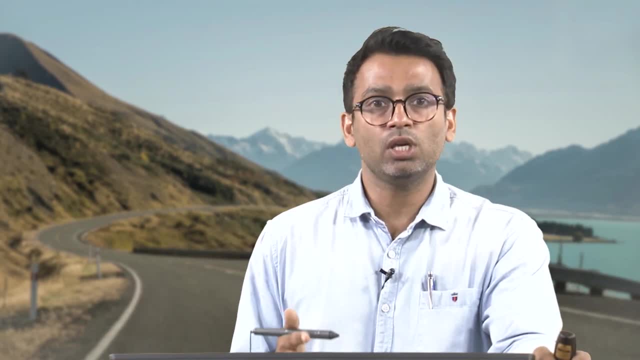 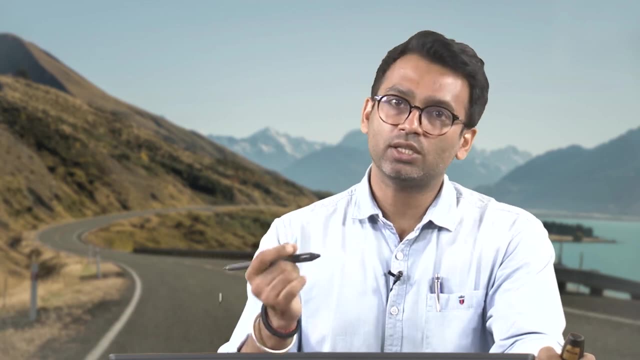 temperatures acceptability of that particular mixture. For example, granular materials. the properties are not very sensitive to the change in temperature So I might not be very interested to see the variation in properties by doing the test at different temperatures in the laboratory. i will do the test only at a standard temperature and that should be sufficient. 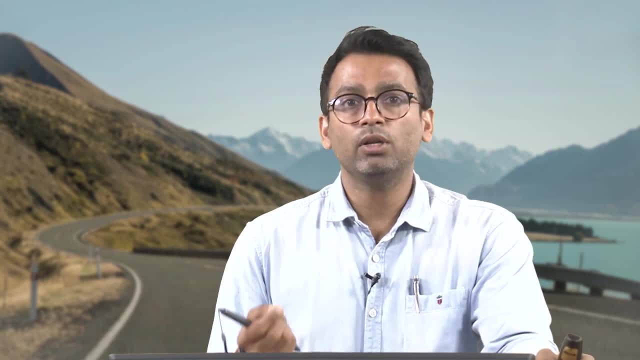 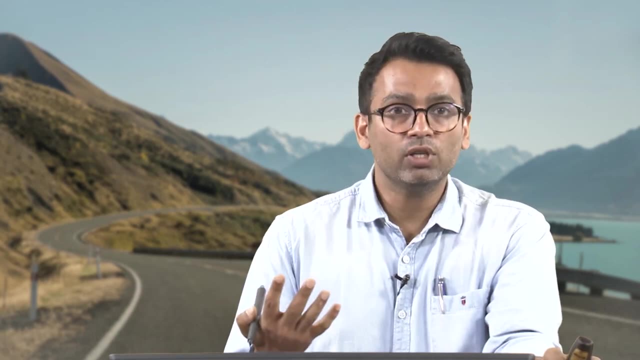 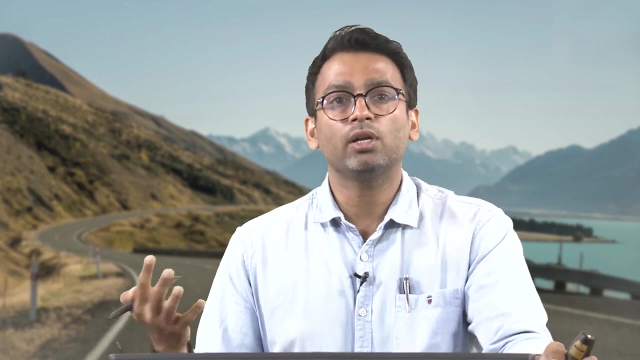 to tell me about the properties. but for soils, for example, though temperature may not be an important parameter, moisture content is an important parameter. so i am interested to see the behavior of the soil at different moisture content. the same is not true when i am talking about a bituminous mixture. i am not going to vary the moisture content. 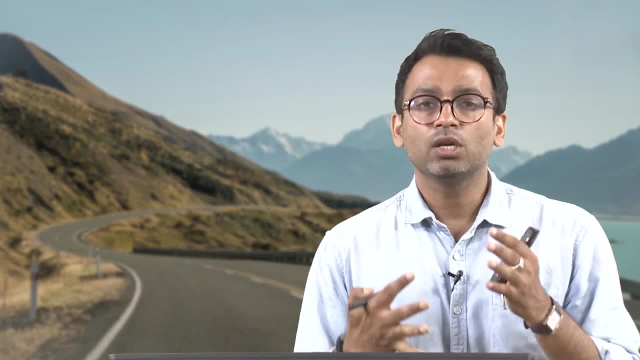 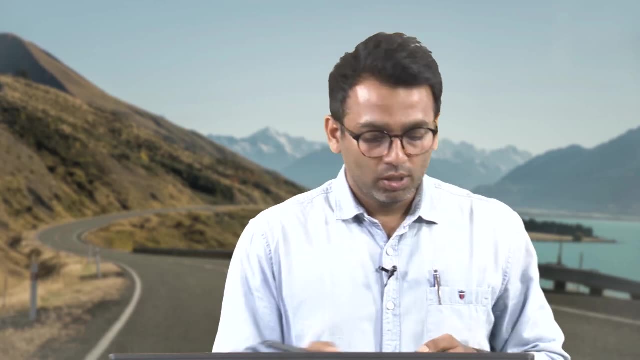 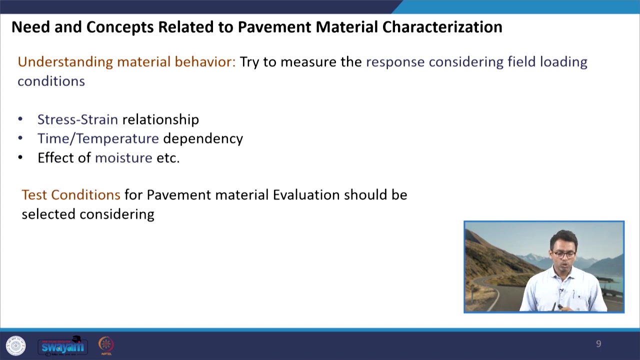 ah, to see how the material response, because that is a dense mix, the properties of the material does not considerably change with change in levels of moisture. all right, so these important points we have to remember while we are thinking about characterizing the pavement material in the laboratory. so finally, we can say that the test conditions 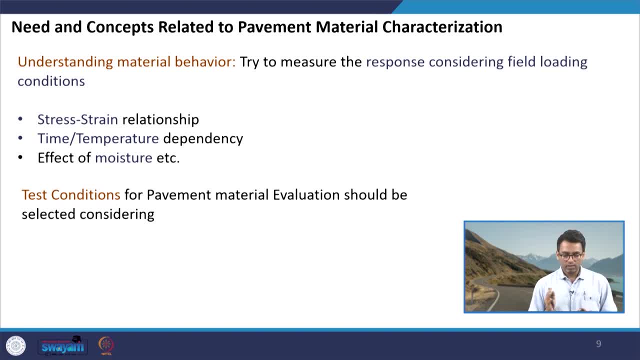 for pavement material evaluation should be selected considering the magnitude, time, frequency and nature of the load. we should know the temperature to the which to which the material is subjected in the field and, accordingly, the temperature should be selected. we have to select the moisture levels depending on the rainfall in that area. 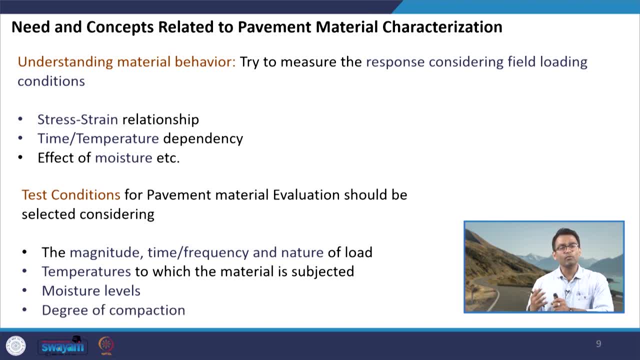 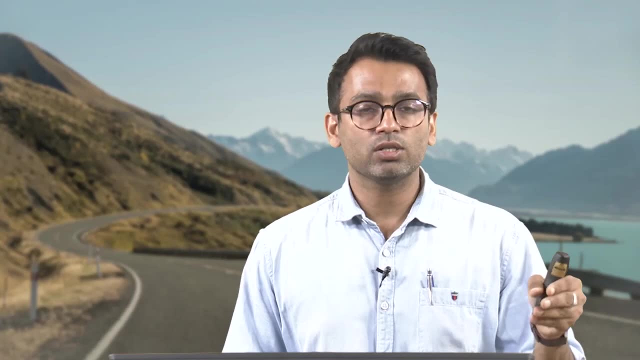 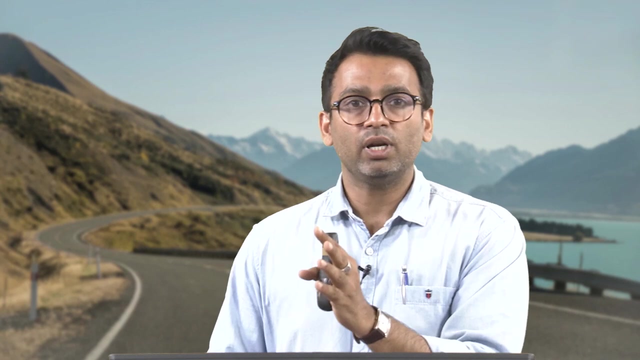 depending on the water table in that area. we also have to ah select the degree of compaction ah depending on the field density conditions we are anticipating. so all these factors have to be considered while doing the ah laboratory evaluation, because the results of laboratory evaluation is going to influence, finally, my pavement design. and once the pavement design. 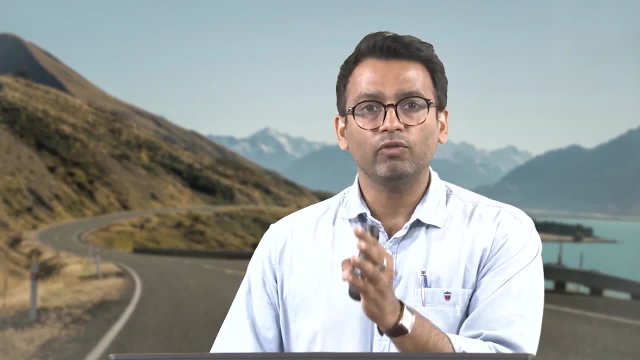 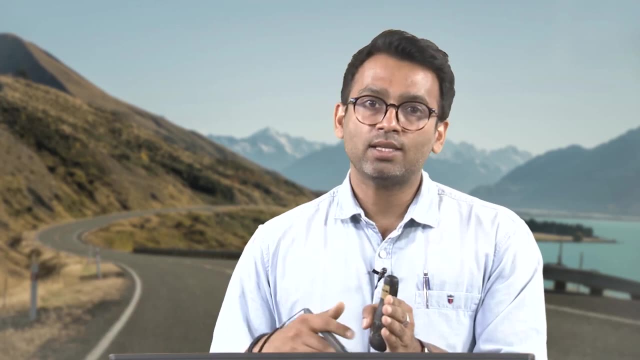 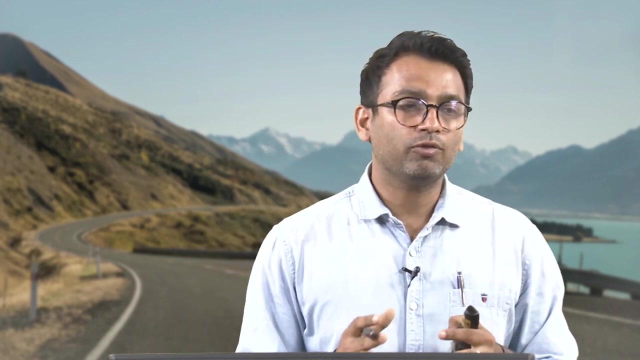 is done, then we have to be very confident that this pavement design, which i have done for a targeting for a specific design period, should perform as i am anticipating it to perform, because you know, ah, this requires a a lot of effort in the laboratory, a lot of testing. 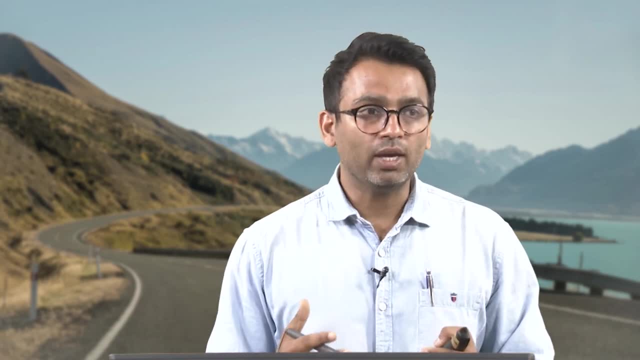 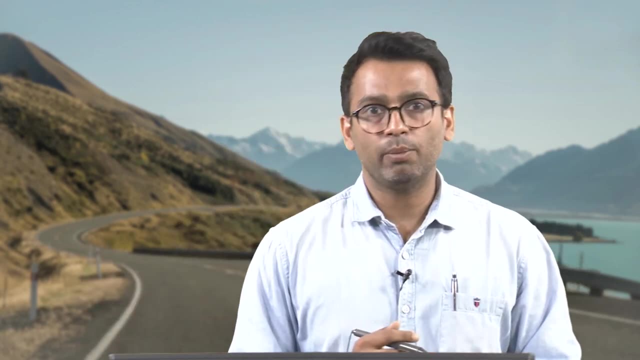 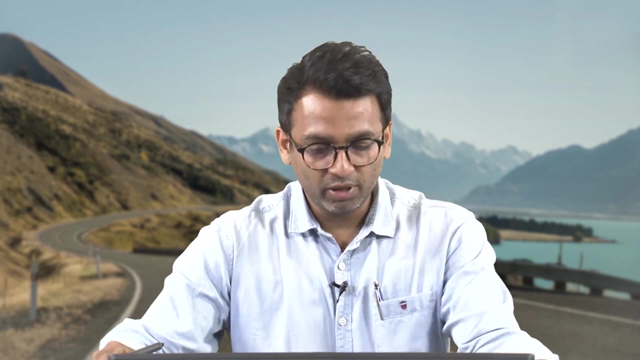 a lot of use of materials, so we have to think about optimizing the the time, optimizing the use of machines to characterize the lab- ah, you know, the samples in the laboratory, ok, so, ah, with this ah background on, ah understanding the importance and need of studying pavement materials, let us start discussing about the first pavement material. 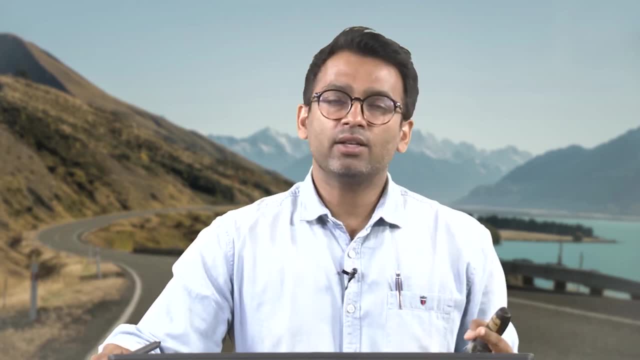 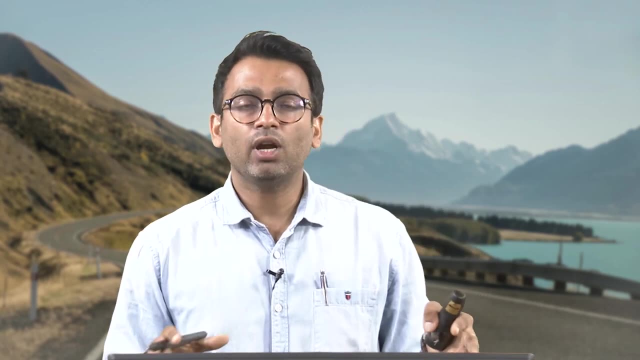 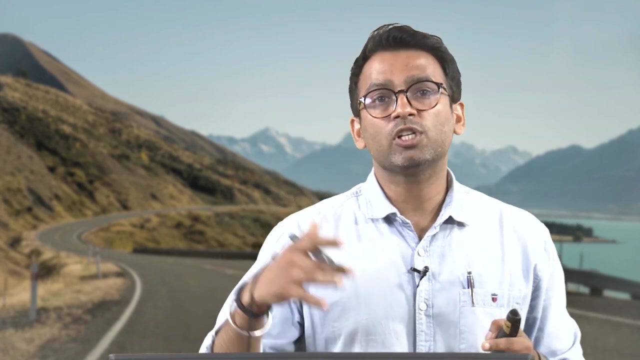 in our list, and that is soil. we will start by understanding soil more as a pavement material, because soil- mechanics anyways- is a very vast subject and we are not going to discuss in detail about all the concepts, ah, you know, related to the ah soil from the perspective. 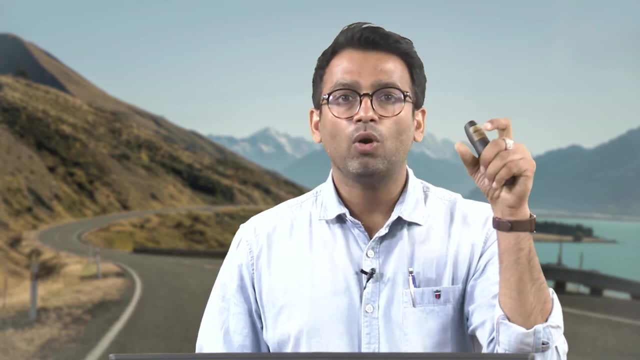 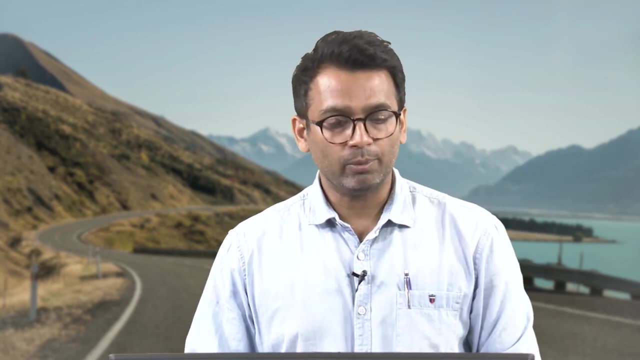 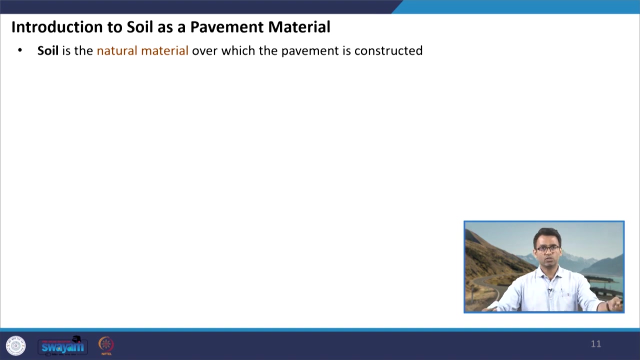 of soil mechanics. rather, we will focus our discussion on understanding the soil, on understanding the properties of the soil ah from the perspective of using it as a pavement material. so soil ah can be defined as a natural material over which the pavement is constructed. so this is the simple definition of soil, considering that we are going to use it in pavement construction. 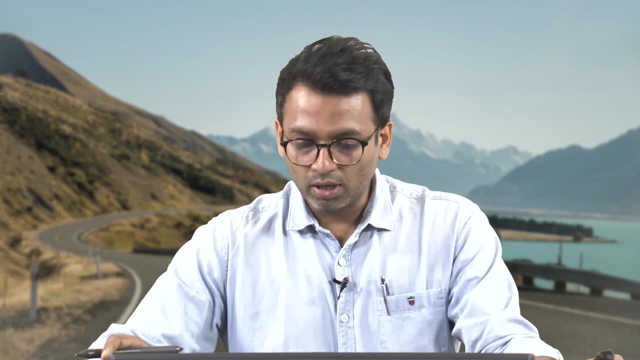 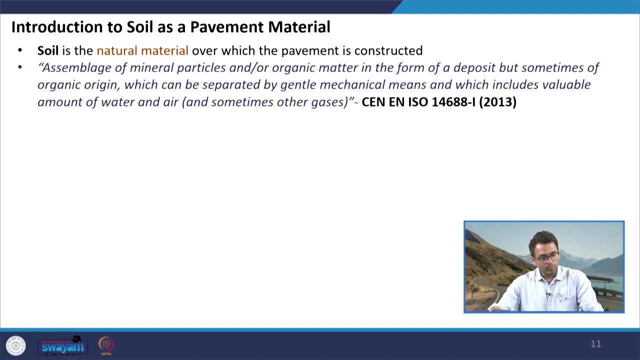 So, if you see the definition given ah in CNENISO 14688, ah, the definition states that soil is an assemblage of mineral particles. now, these are some critical words. which tells us: you know you. which which gives us much indication about the ah, you know properties. 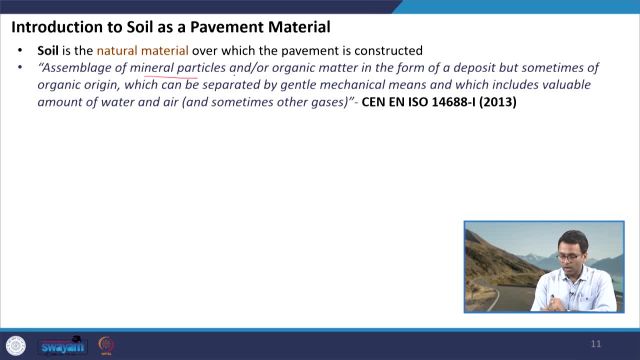 of soil. So it is an assemblage of mineral particles and or or organic matter, in the form of deposit, but sometimes of organic origin, Which can be separated, which can be separated by a gentle mechanical means and which includes valuable amount of water and air and sometimes other gases. so this is a definition ah placed. 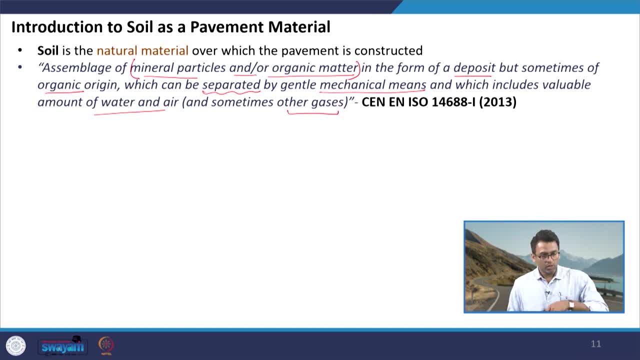 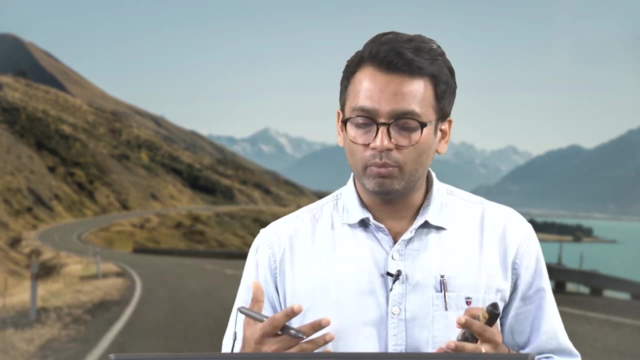 by ah, this particular ah specification, and it tells us that soil basically consist of minerals. it can consist of organic matter, ah, mostly it. it appears as a bulk, but it can be separated by using, you know, ah, ah. So by through mechanical means, by subjecting the sample to mechanical forces and soil in 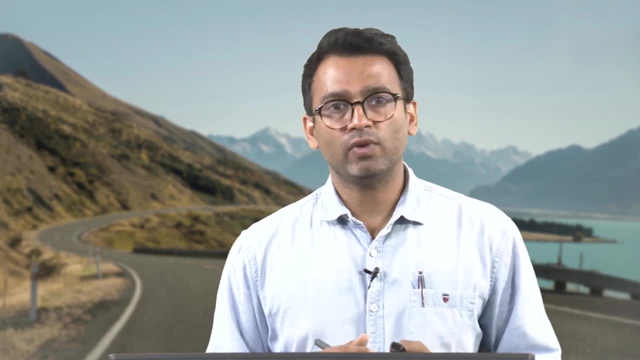 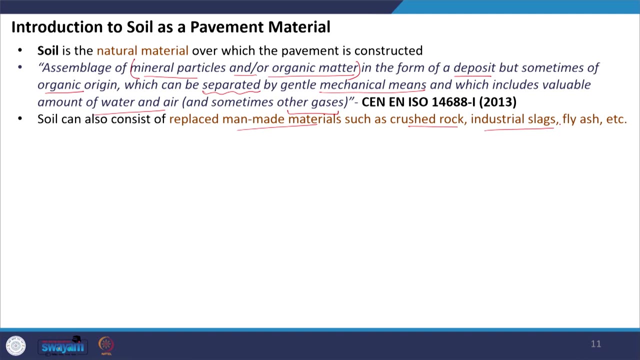 general, it contains certain amount of water, as well as air, if you see the volume of the soil. In addition to the natural soil, it can also consist of replaced manmade materials. for example, we can have crushed aggregates, crushed rock, we can have industrial slags, we can have. 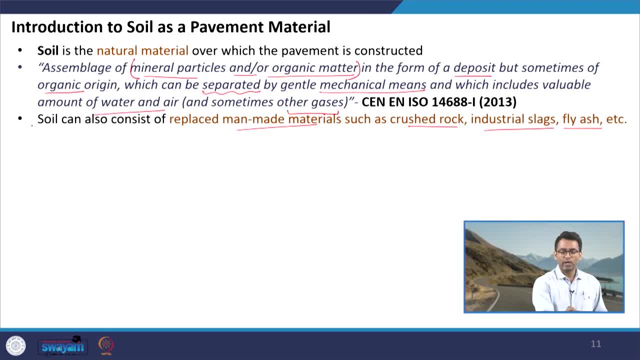 use of fly ashes, etcetera. ok, So the soil which I am going to use as a foundation layer in the pavement- So this is what I am referring to here- It is primarily formed by disintegration of rocks or decomposition of vegetation. 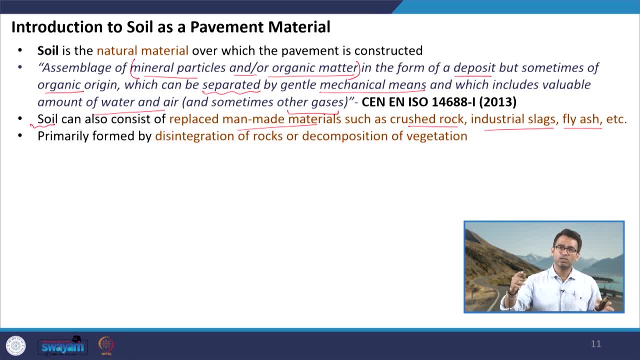 So the existing rock which is there at the surface. it can decompose over a period of time. let us say this is the existing rock, So the top layer will decompose over a period of time. this decomposition can be due to weathering action. 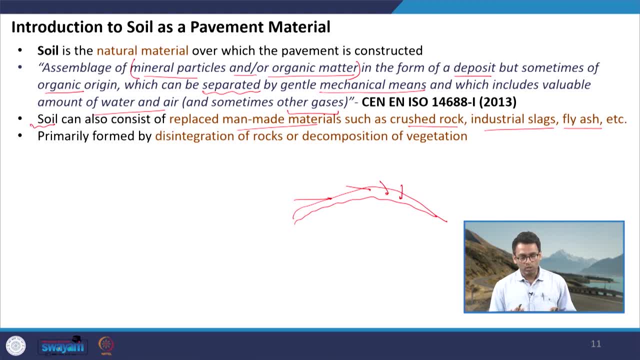 So movement of water can be due to chemical action and so on, and for a considerable period of time. So this top layer, it becomes weak, it changes its mineral composition, it changes its physical nature and it gets converted to a new material which we are, ah, denoting as soil. 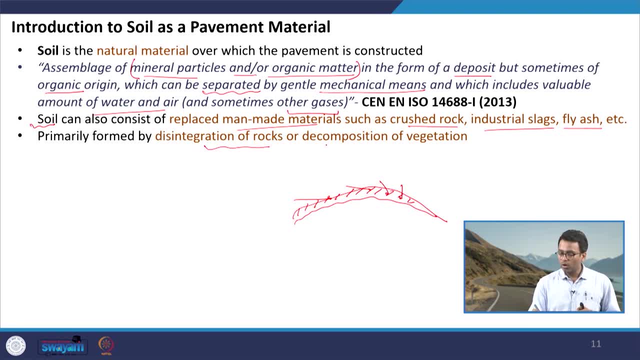 So it can be formed by disintegration of rocks or decomposition of vegetation. also, the existing vegetation can decompose and it can take the form of soil And these are like organic soils Now if you talk about the categories ah of soil. So these are few categories which can be listed. 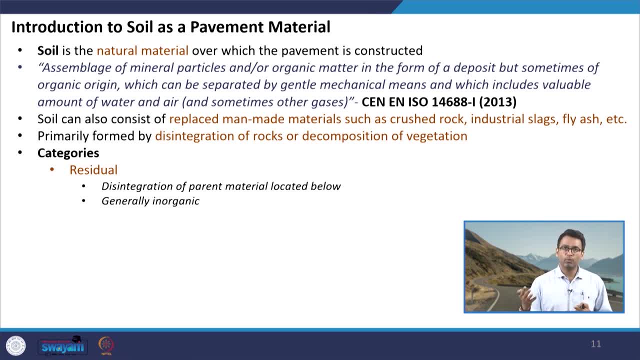 So we have residual soils, as I mentioned. these are from the disintegration of the parent material, which is just located below, and it is weak in nature in comparison to the ah parent material. ah, It is generally inorganic in nature because it is coming from the ah rock as the parent. 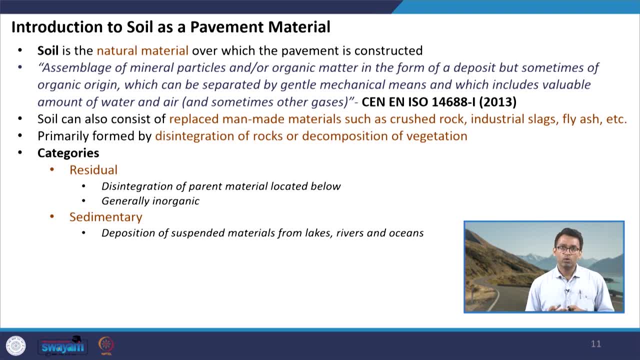 material Now, sedimentary deposits, which can be of ah, which can be in the form of suspended materials from lakes, rivers and oceans, For example, you have alluvial soils, you have marine soil. So alluvial soils are, you know, better in comparison to marine soils, if you see them. 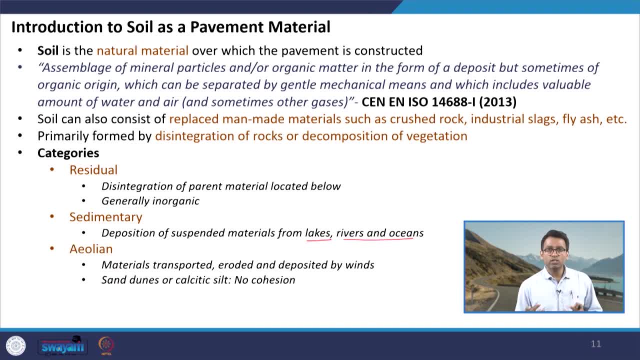 as a construction material. ah, We have aeolian soils, which comes to movement of winds, So these are material transported, eroded and deposited by winds, For example. we have sand dunes, we have calcitic silt. So this, these materials usually, for example, sand dunes, they do not.